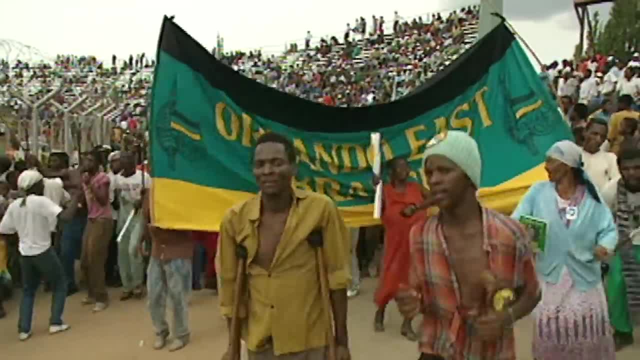 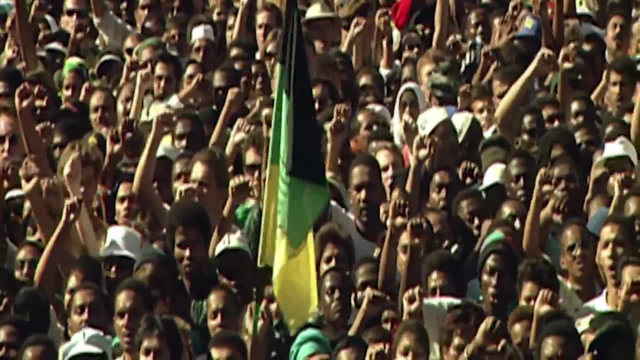 South Africa could be the poster child of the potential of African economic and human development If the white and black nations could truly integrate into one. the country was well on its way towards being considered a social and economic equivalent to, say, New Zealand. 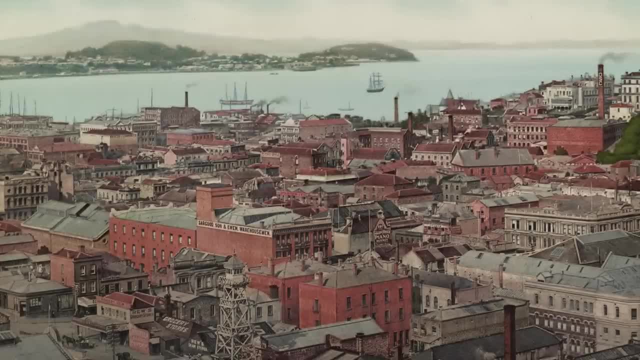 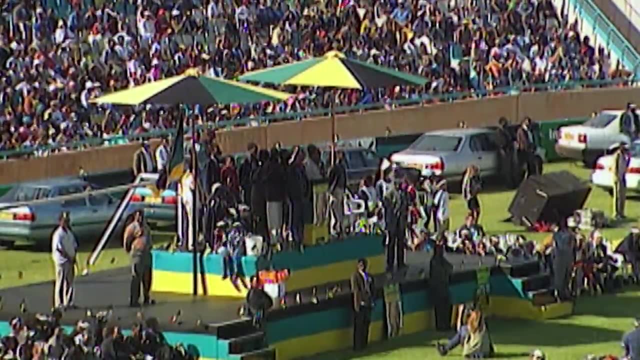 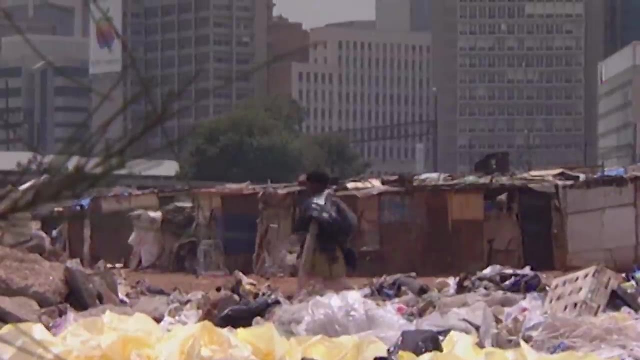 another former British colony in the southern hemisphere that managed to transition into a self-sufficient, high-income multicultural society. Crucial to this, perhaps the greatest task that Mandela and his ANC party was faced with was how to build a black middle class. The legally enshrined systems of segregation were 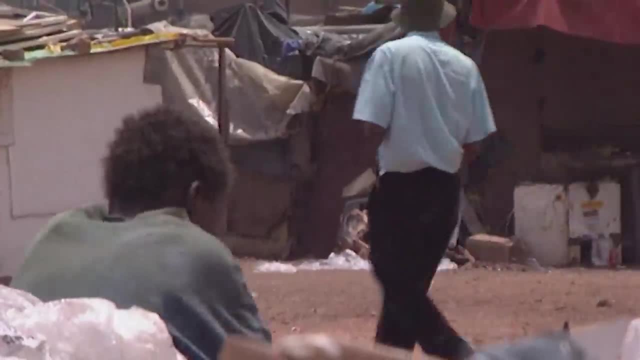 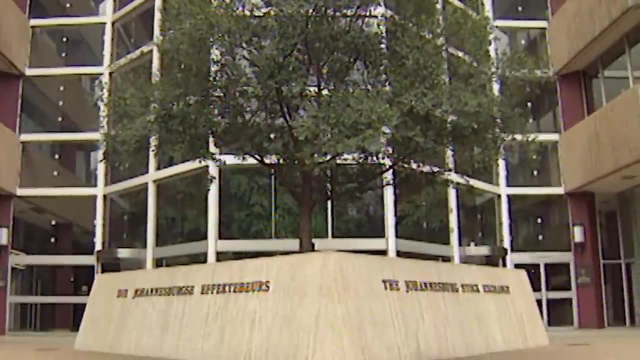 easy to do away with—they could be reversed in an instant—but what was left was a massive population trapped in the cycle of poverty. Simultaneously, there was the wealthy white population at the center of the current economic system, who would not tolerate a similar system of segregation. They would not tolerate a similar system of segregation. 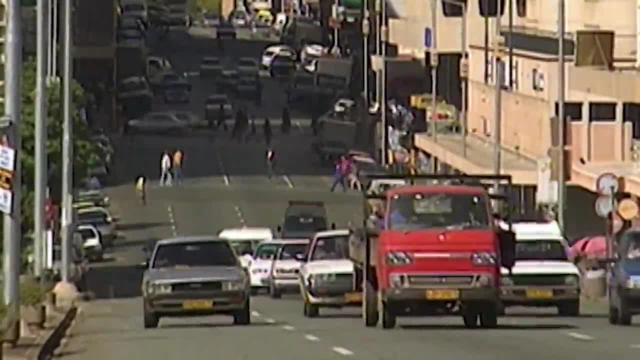 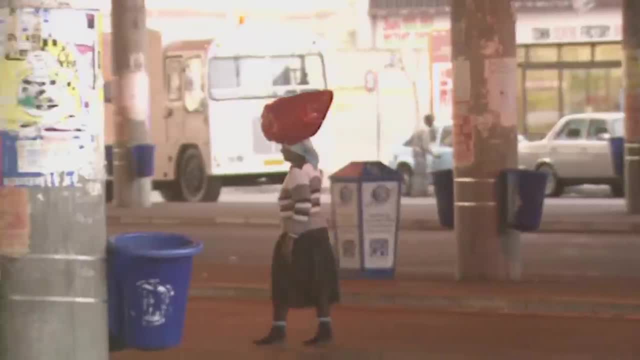 nor would they tolerate a simple redistribution of wealth. So the ANC had to thread the needle—correct for historical wrongs while maintaining most of the status quo. Initially, they were fairly successful at this. The beginnings came naturally as black party members moved into many of the 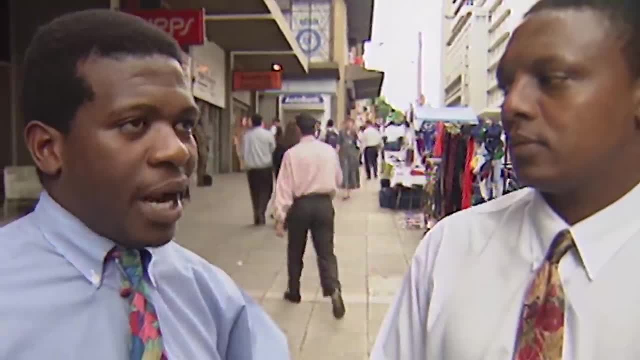 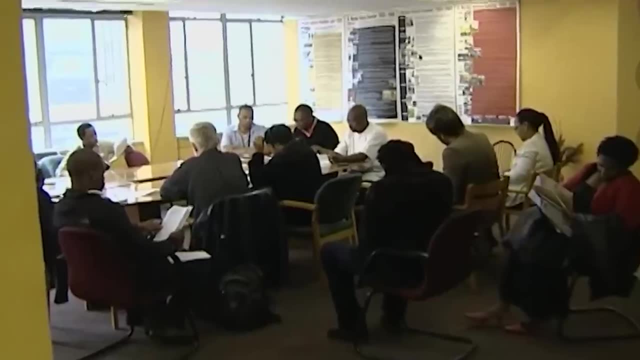 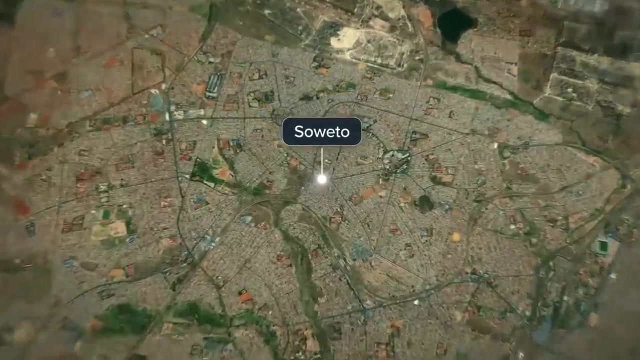 stable, well-compensated public sector jobs previously held by the white minority. then the trend permeated elsewhere, as qualified individuals excluded only due to the color of their skin entered every other newly desegregated profession. Formerly impoverished townships like Soweto metamorphosed from slums into sprawling suburban. 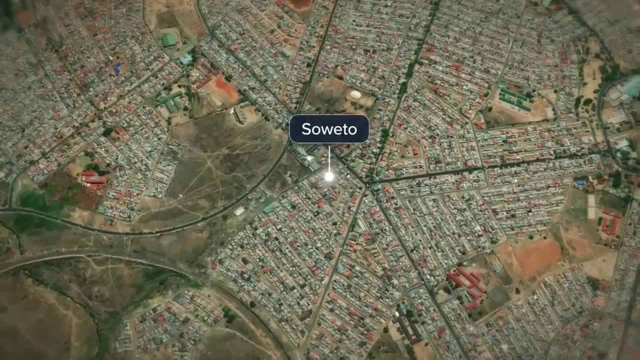 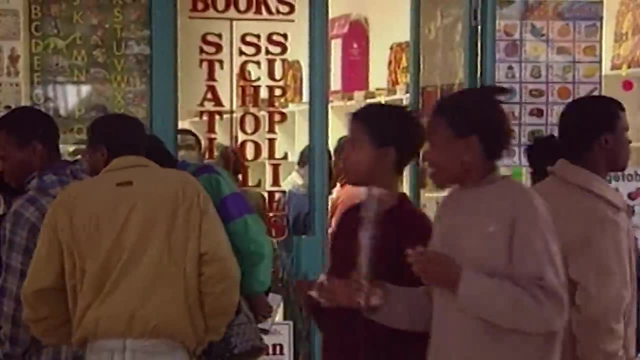 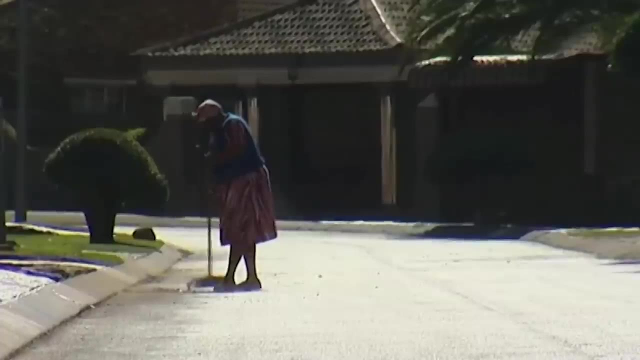 neighborhoods filled with rows of single-family homes and ample assortments of upscale restaurants and bars. And, crucially, this wasn't due to wealth moving in, but rather wealth being built—the white population of Soweto stayed at just a fraction of a percent More broadly nationwide, according to. 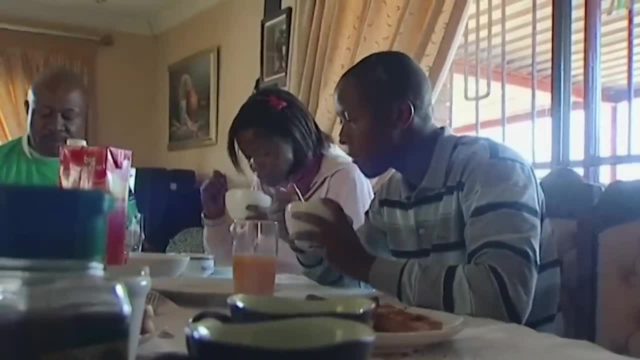 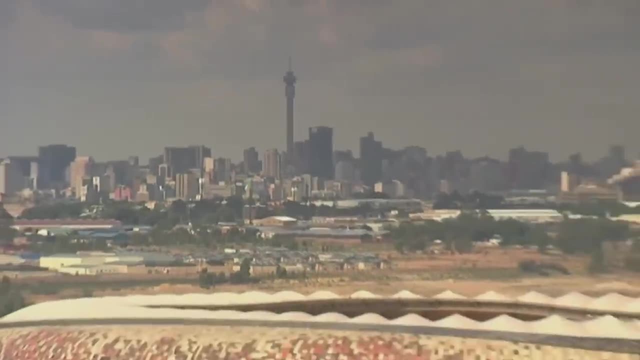 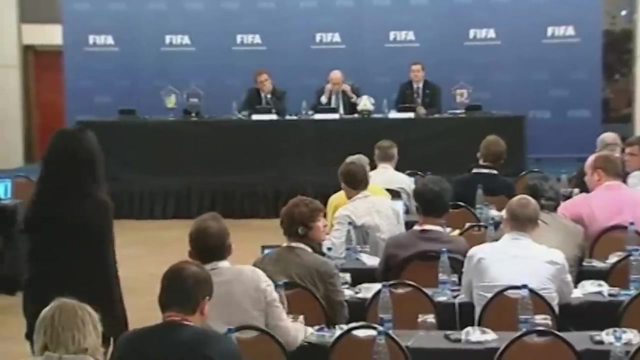 one study's definition, the black middle class grew from just 1.7 million in 2004 to 4.2 million just eight years later. As perhaps the strongest validation of South Africa's progress so far, the nation was selected to host the 2010 FIFA World Cup—a never-before-seen event on the African. 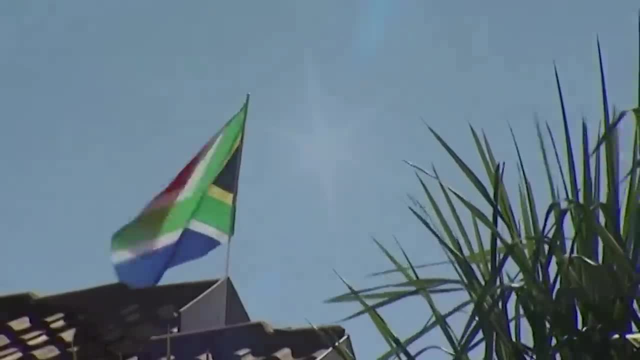 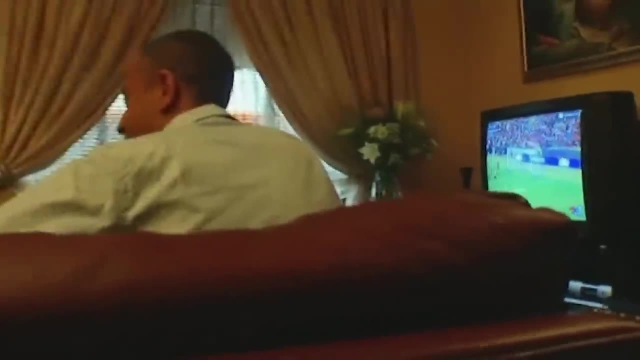 continent. This sent a message—it said that, of anywhere in Africa, South Africa was the place most capable of hosting the world's second-highest-profile sporting event. Inevitably, naysayers arose. They said the nation couldn't possibly build the state, but could in fact build. 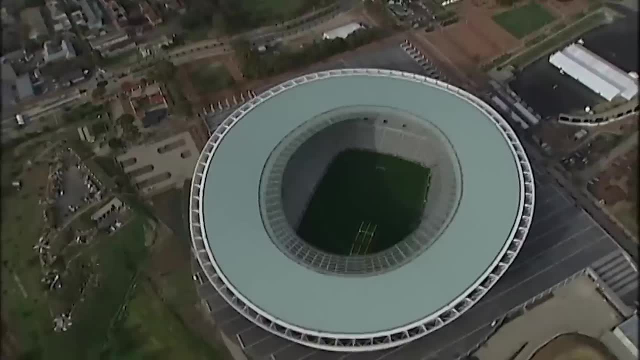 its own sport in the region, In shortiyet, had to leave the nation to change its course. They said the stadiums in time. then when they did, they said the stadiums were shoddy and would crumble apart. then when they didn't, they said that fans wouldn't possibly show up. 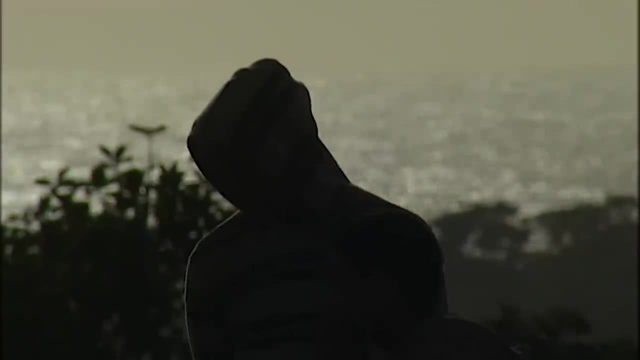 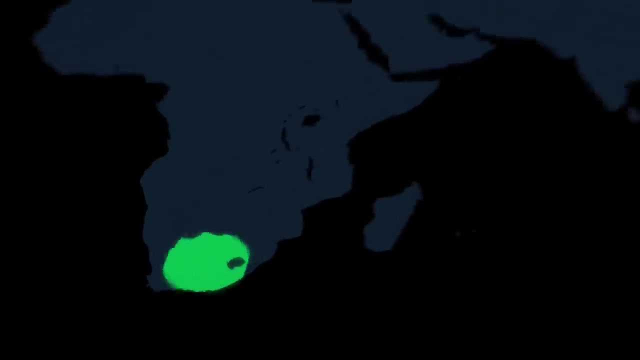 fearful for their lives in crime-riddled South African streets. but they certainly did. As the sound of Vuvuzelas engulfed the TV broadcasts, the world was captivated by the host country, and it was now thought of in the same vein as Germany or Japan or France. 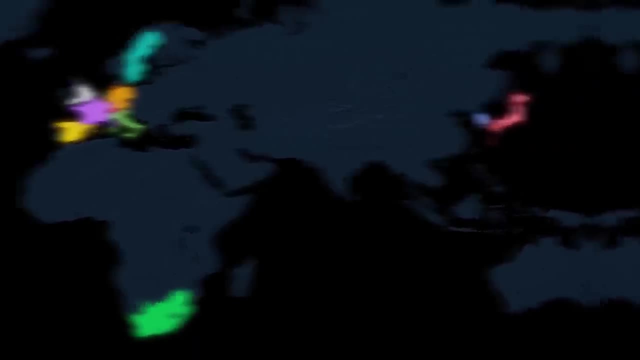 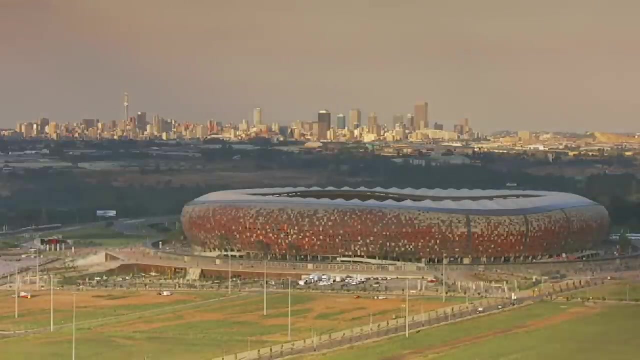 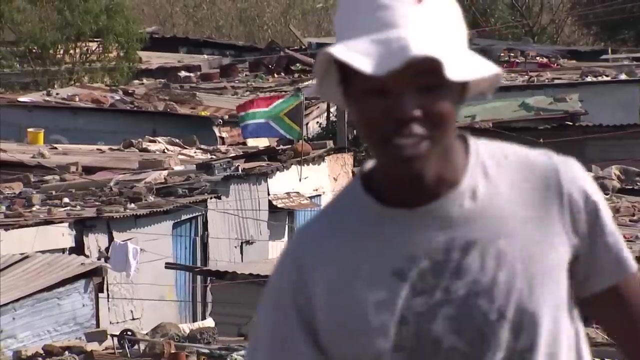 or any of the other World Cup hosts. But eventually Spain bested the Netherlands. the TV broadcasts wrapped up, the lights of Soccer City Stadium switched off, the fans flew home. the years marched on and time revealed an uncomfortable truth. While the government was able to emulate stability for the short period they were able to create, 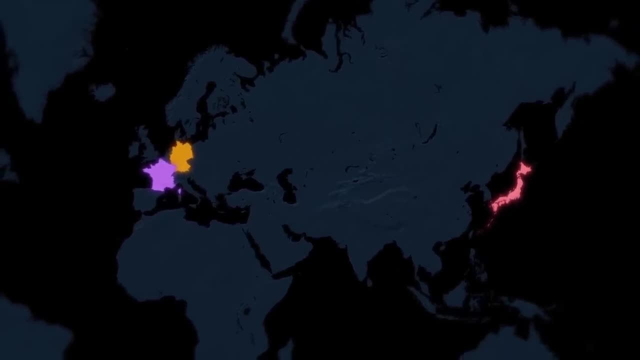 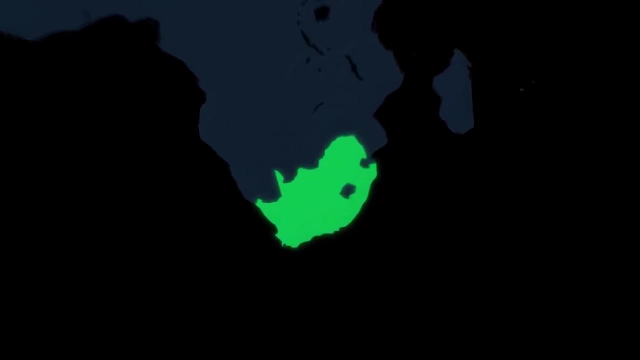 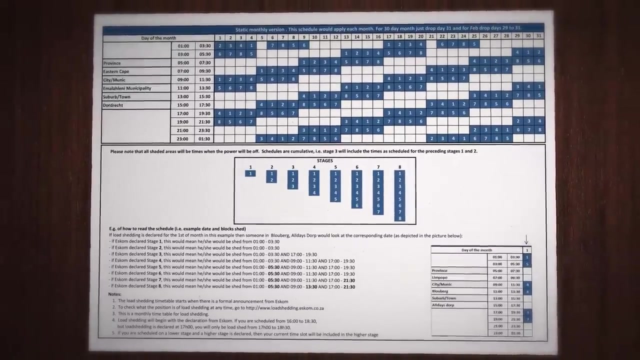 a facsimile of the experience in Germany or Japan or France. it didn't last. Progress had stagnated. It might have actually reversed. This is perhaps best represented by this, the least popular document in South Africa. Nowadays it's published each month by the government-owned power utility ESCOM, and 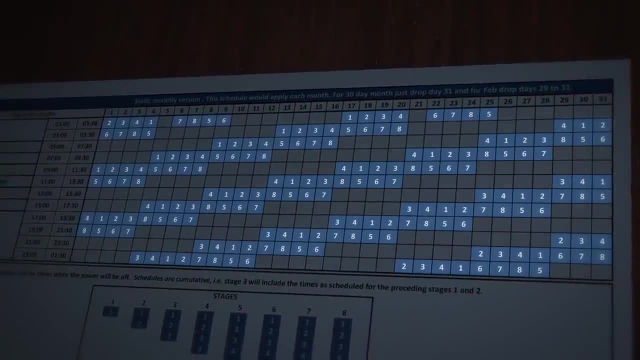 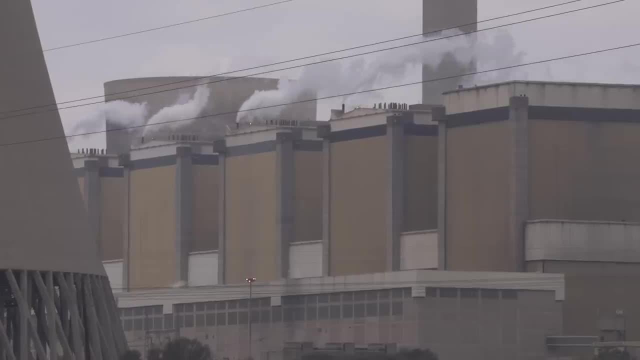 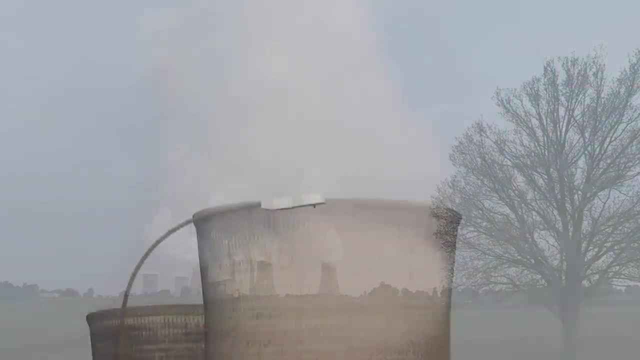 it outlines the schedule of when each municipality will have their electricity supply shut off. After decades of deferred maintenance on a power system mostly designed to service the white minority, plant failures have escalated this issue into a chronic mismatch between supply and demand That creates this dissonance. 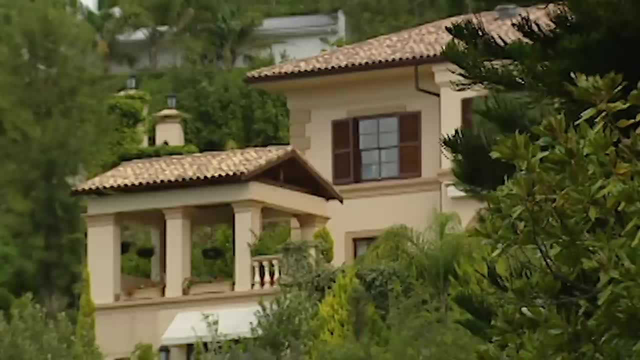 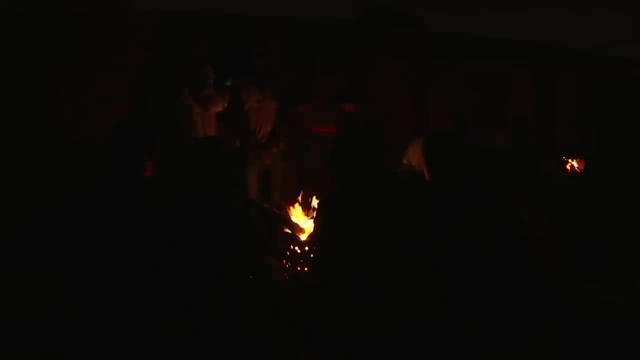 This, in parts, looks as developed as the most upscale areas in Europe, yet is plunged into darkness as frequently as its poorest African neighbors. These days, a lack of load-shedding is the exception—so far in 2023, there have been 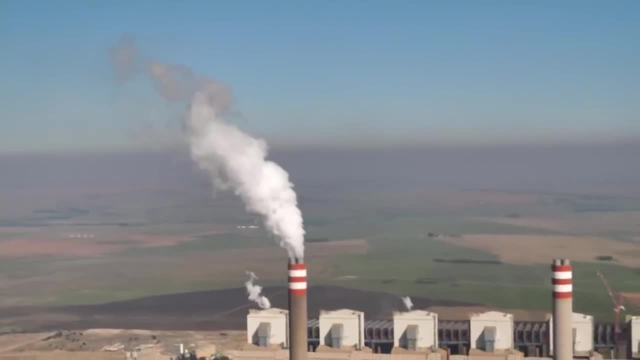 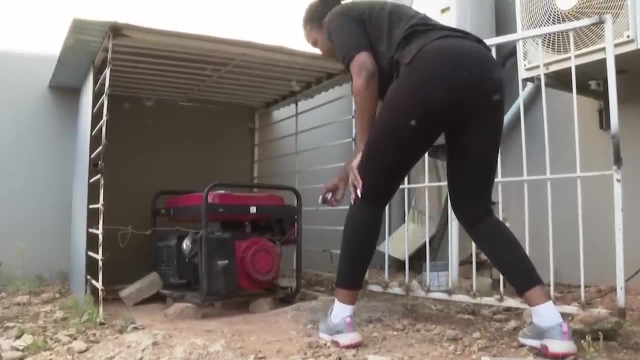 5,858 hours when the grid has failed to meet demand. But while perhaps the most palpable issue that creates some of the most sizable domino effects, South Africa is increasingly failing to provide the absolute bare minimum of power. It's not just the power of electricity, it's the power of electricity. 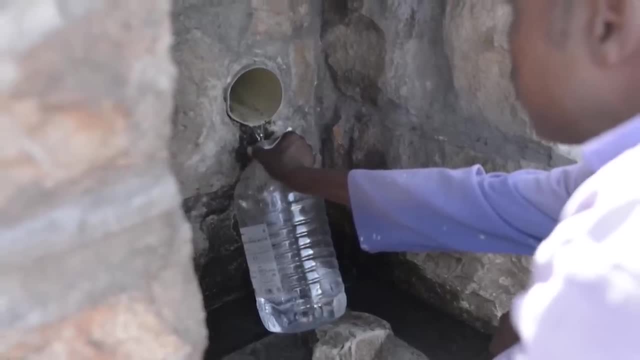 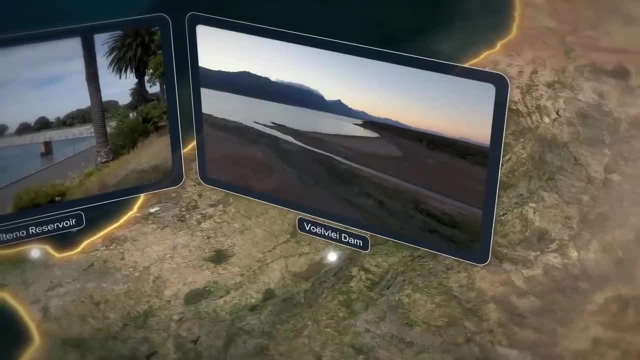 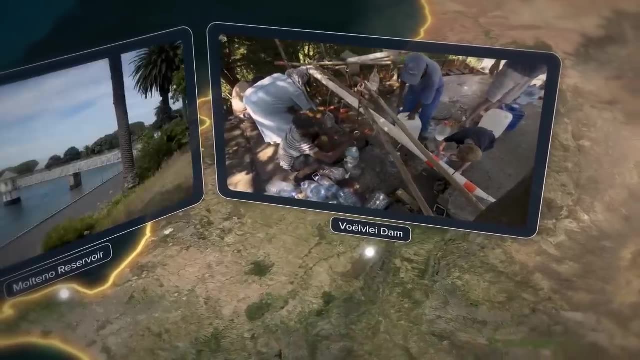 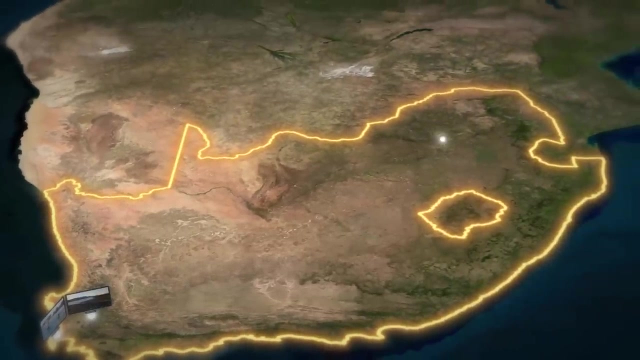 the city's reservoirs ran dry during a drought—a crisis created in part by a lack of government foresight—but, more broadly and regularly, the share of households with access to drinking water has started to decline in recent years. Water infrastructure is crumbling and just recently, dozens have died on the outskirts. 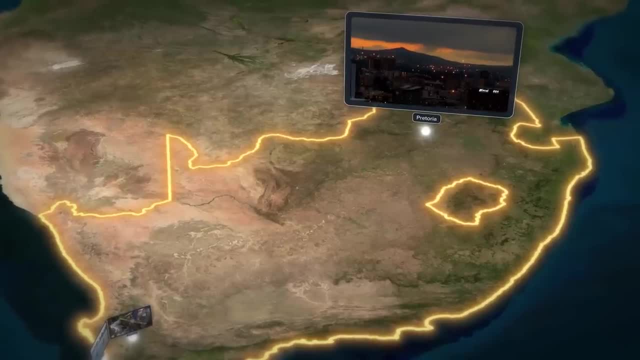 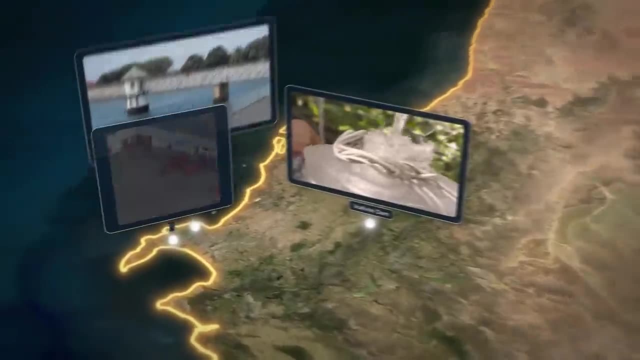 of Pretoria, the administrative capital due to the economic pressing of the country's, to cholera, a disease virtually eliminated from the modern world thanks to modern sanitation systems. The nation's homicide rate is skyrocketing, climbing up towards its all-time high, and 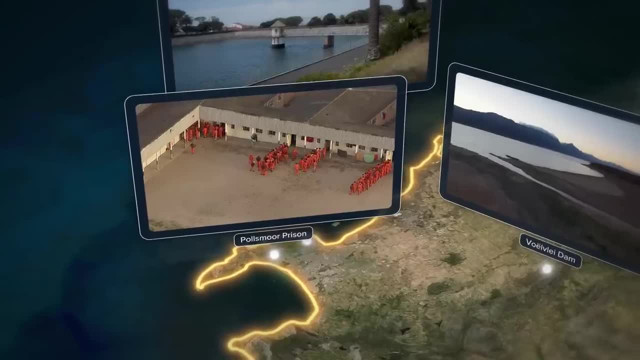 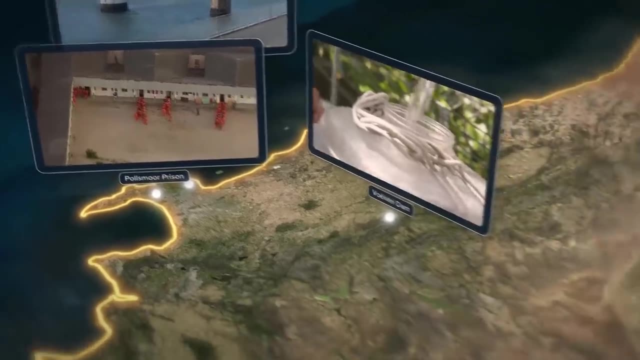 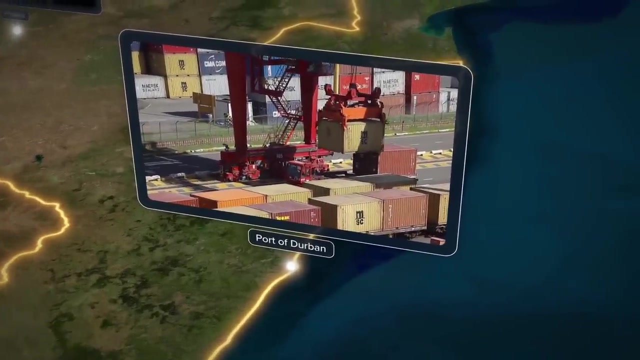 the police and judiciary appear entirely ineffective at combating this, as just 20% of murderers end up with anyone in court, and even then, just 31% of the public has trust in the courts. as the legal system breaks down as well, South Africa's state-owned freight rail monopoly, Transnet, is too collapsing. 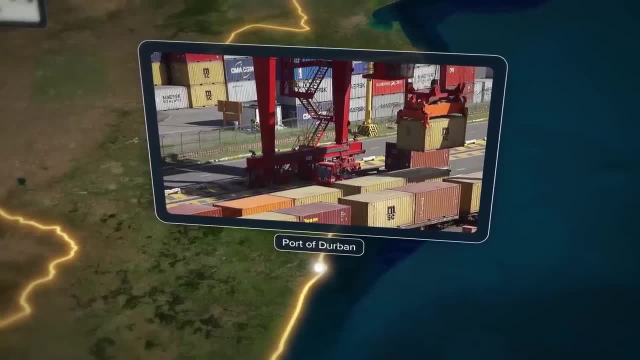 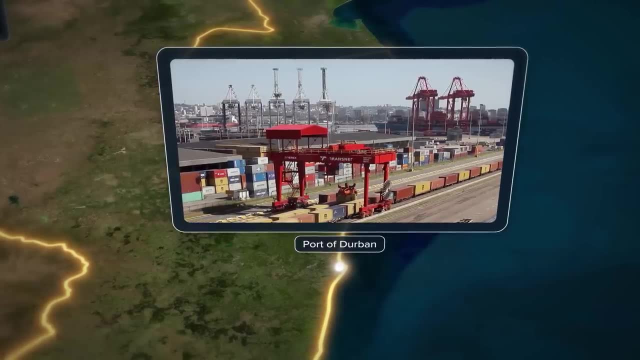 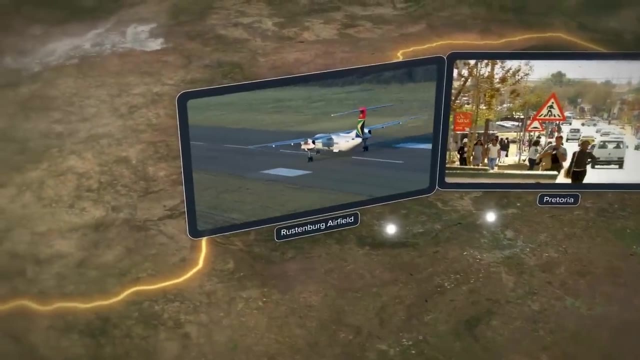 In a very similar situation to ESCOM, as it closes lines, struggles to keep locomotives running and carries 25% less cargo today than in 2015—a massive constraint for the country's lucrative, export-focused industrial sector. South African Airways, which was separated from Transnet in 2006 but remained government-owned, 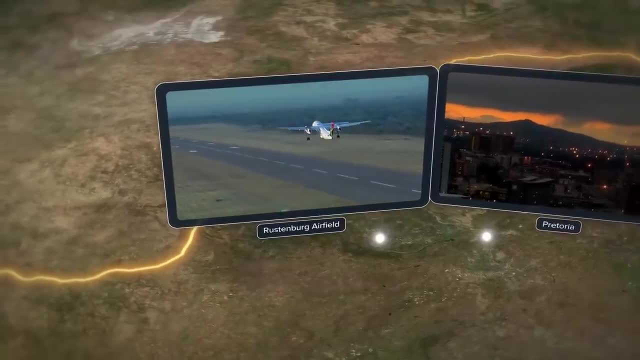 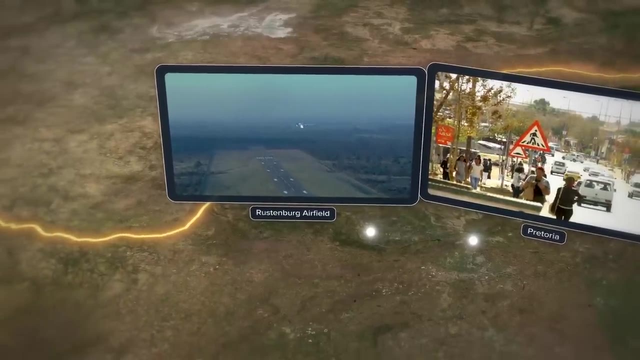 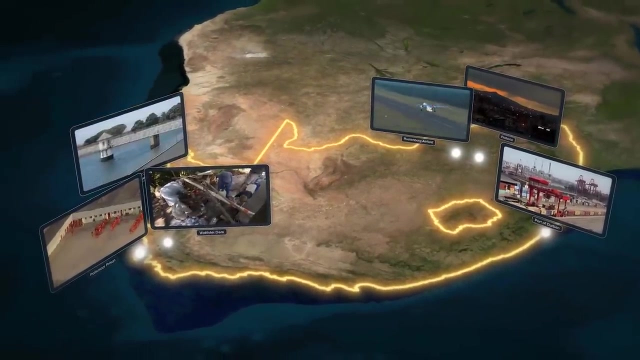 fully collapsed and ceased all operations in 2020, before restarting with new financing as an embarrassing shell of its previously globe-spanning self. No matter where one looks, one struggles to find any case where government service is improving in South Africa, and the closer one looks, the more sense this starts to make. 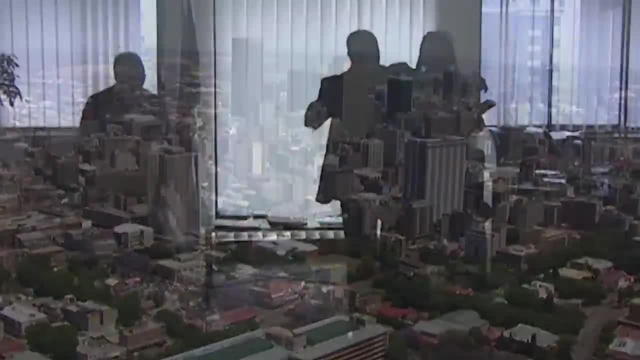 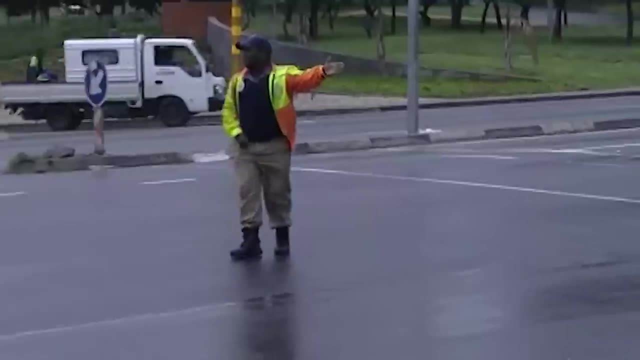 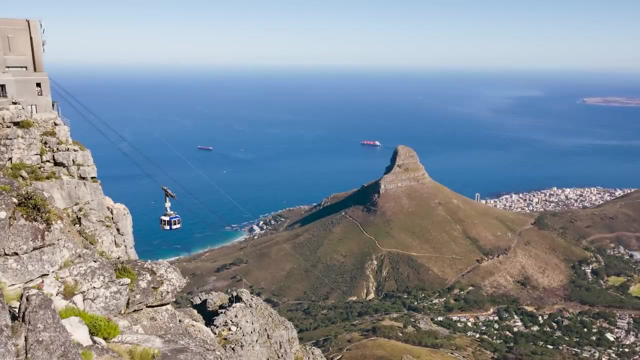 When the blackouts began in 2007,, they were little more than random, local, short-lasted, inconvenient irregularities. Then, in the January heat of the southern summer, they got a lot worse. With demand surging past supply, tourists sat stranded in cable cars high above Cape. 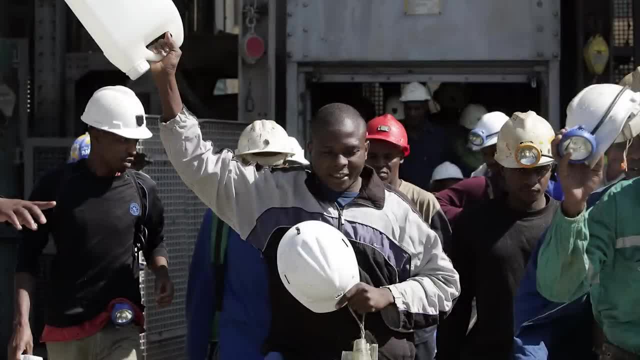 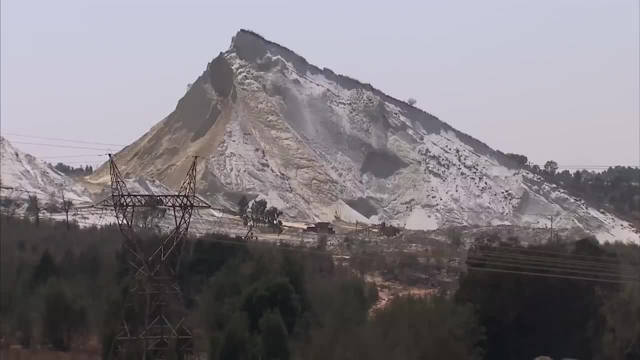 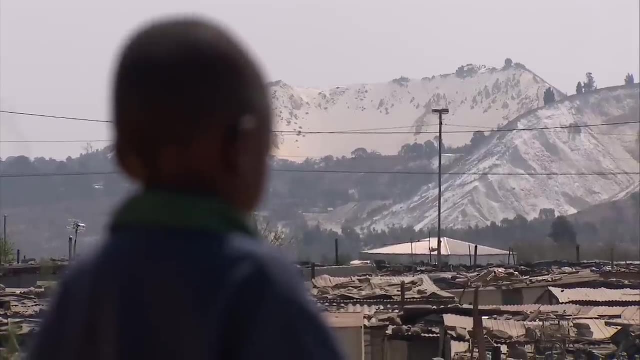 Harbour mines, evacuated miners from shafts that they could no longer ventilate or cool, and the South African government declared a national emergency. The panic power cuts made international news and tipped global markets, as the price of gold and platinum shot skyward after announcement that mines might not open for another six. 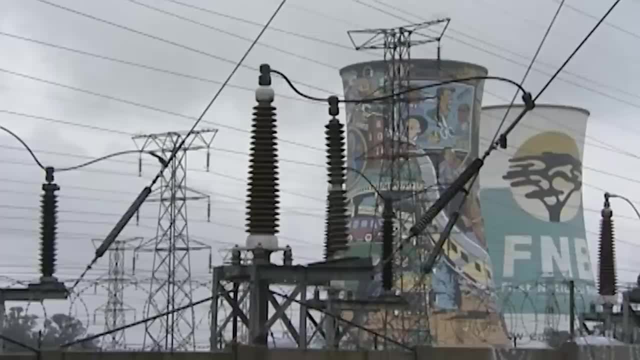 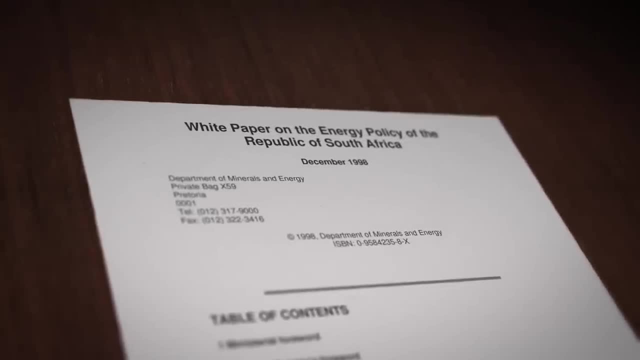 weeks. It was not the first load shedding that ESCOM had mandated in recent months, but it was by far the worst, And it was right on time. In fact, this very moment when South Africa's mighty grid was about to collapse, it was 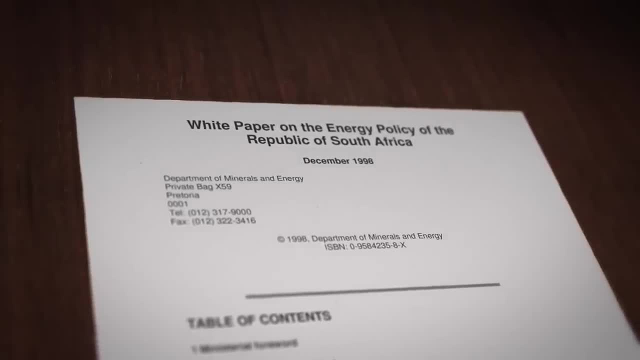 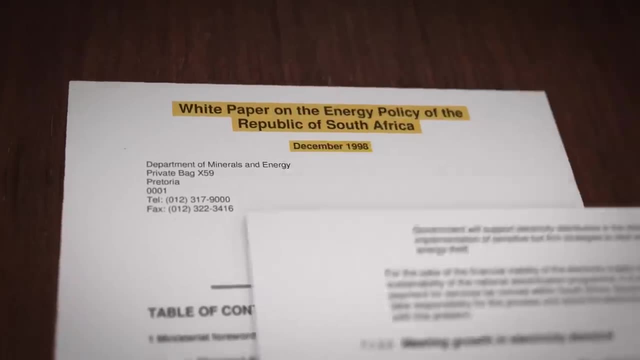 the first time that the grid was catastrophically overstretched by its consumers had been predicted to merely the exact year in this 1998 white paper. As the paper had estimated, should no action be taken to expand power supply in South Africa. 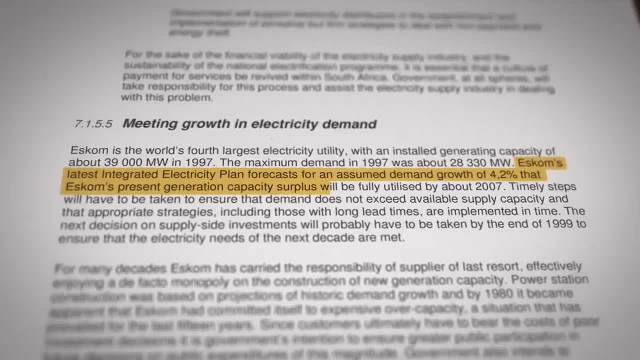 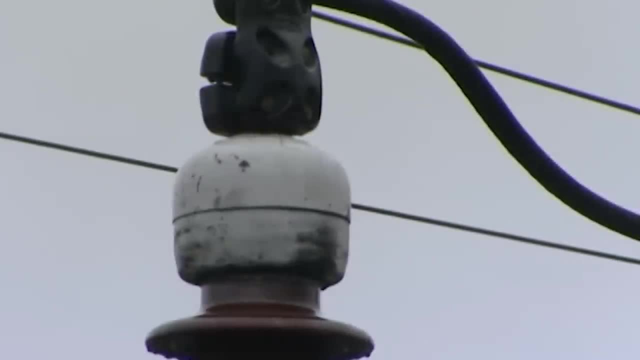 the country's surplus, then sitting at a healthy 25% in 1997, would evaporate away by about 2007.. And no action was taken. For all that changed politically and socially with the end of apartheid and the rise of the ANC, South Africa's grid was still the same. 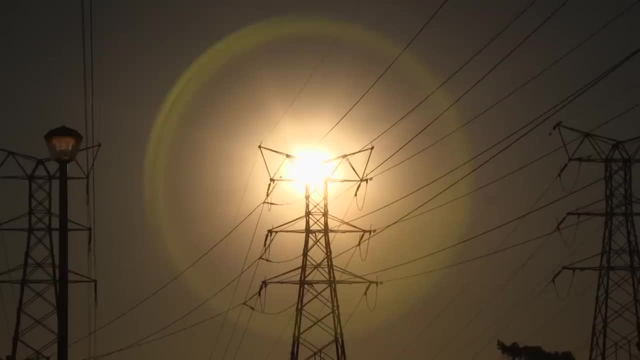 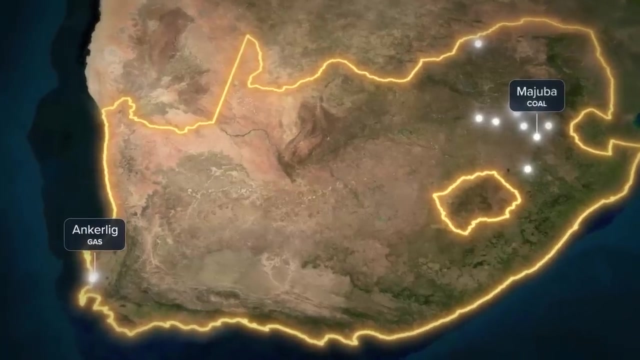 It was still the same. The grid on the supply side just didn't. Of the nation's 15 separate power plants capable of producing more than 1,000 megawatts, only these two came online during the period from 1990 to 2008,. while these two were hastily, 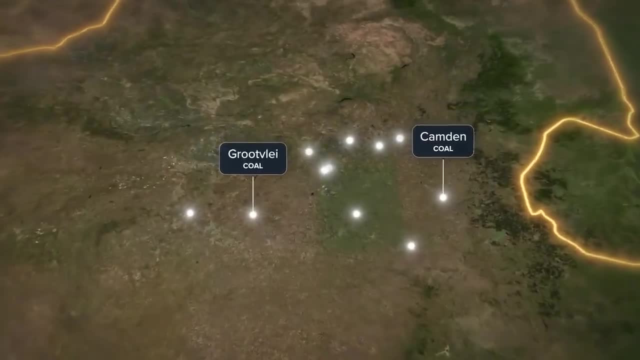 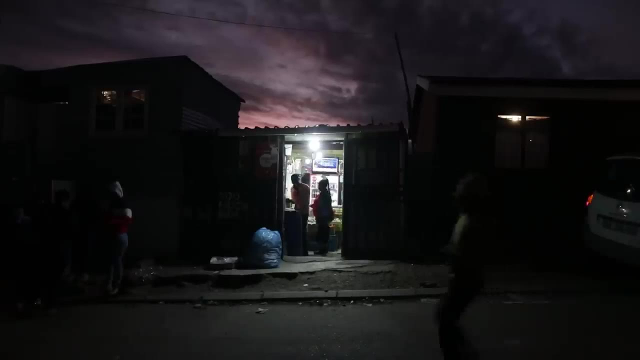 brought back into production, having been mothballed decades prior, when the country was power-flush, As heavy industry moved into the resource-rich country and progressive-minded policies extended the grid to black and underprivileged neighborhoods. post-apartheid, the margin between power needed 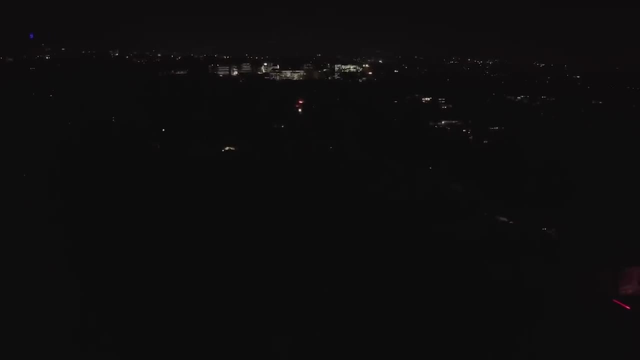 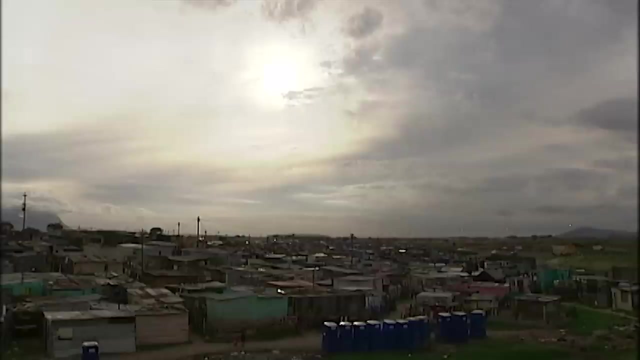 and power-available fell First, shrank, then disappeared entirely. And why South Africa failed to take action is also explained by this white paper. White papers, by their very nature, are supposed to be, if not concise, as concise as possible—outlining. 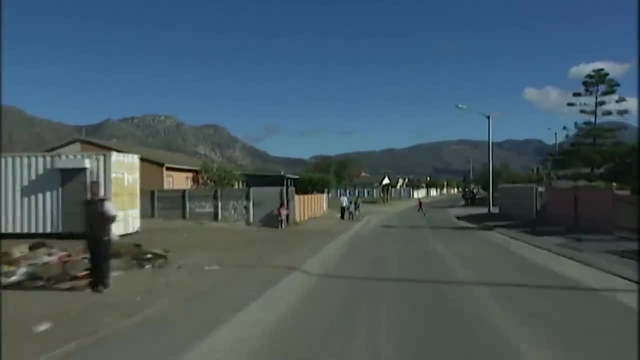 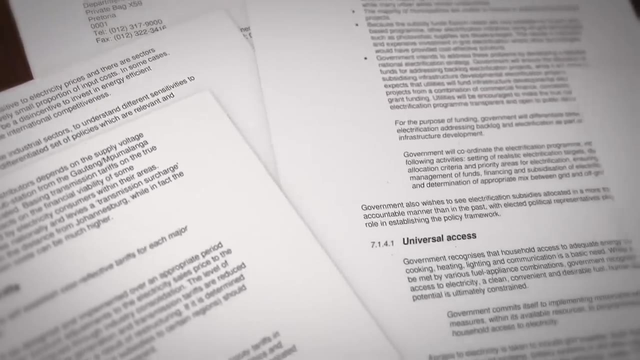 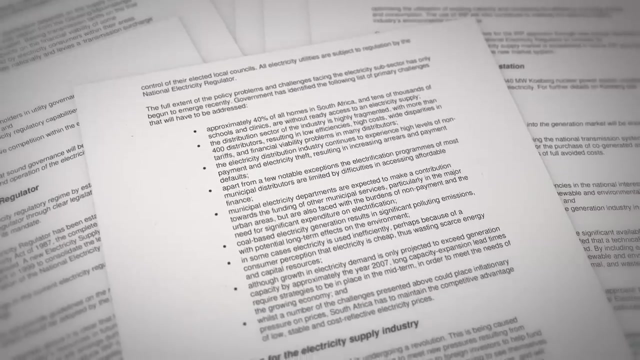 specific problems, providing only the context deemed absolutely necessary and offering a set of specific options forward. This one runs 110 pages, And as for problems specifically facing the supply side, Well, those aren't addressed until 41 pages in when the danger of a potential capacity 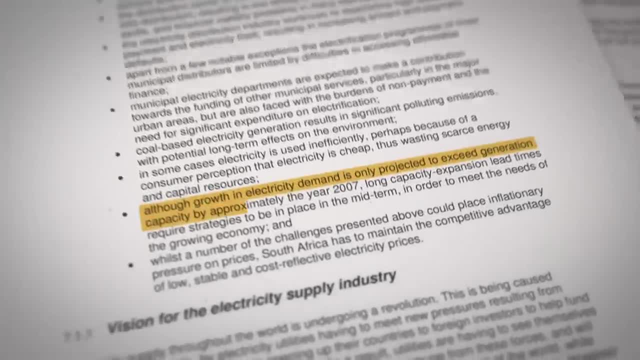 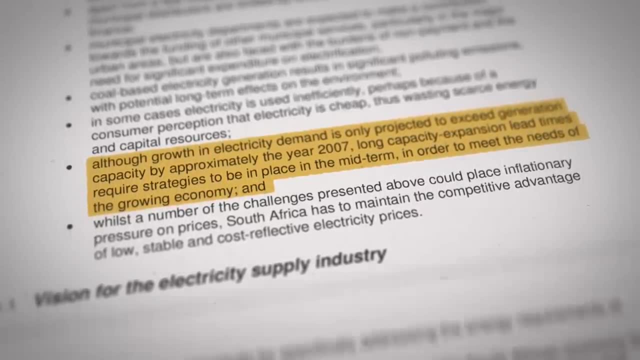 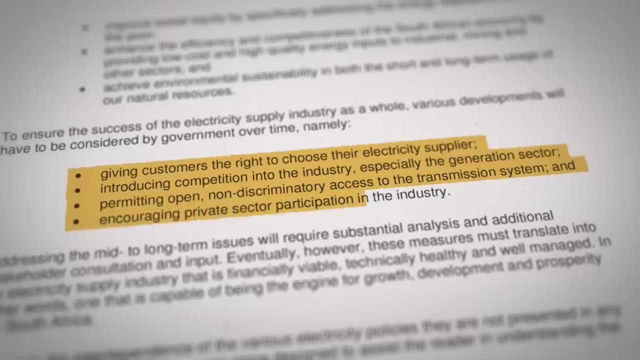 shortage isn't touched on until bullet-point-eight, behind issues of fair access to the grid, environmental concerns and wasteful usage. And as for fixing the problems, there's this—a vague memorandum to expand access and incentivize competition, recommendations both problematically broad and puzzling for. 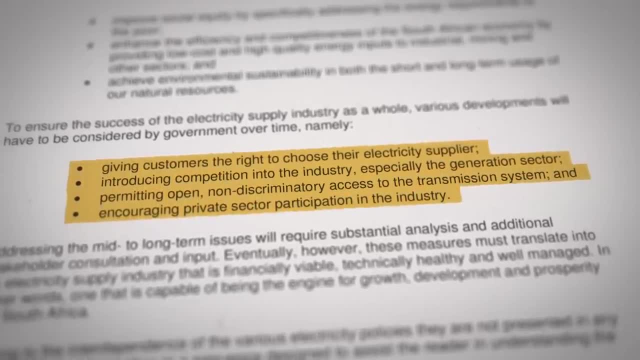 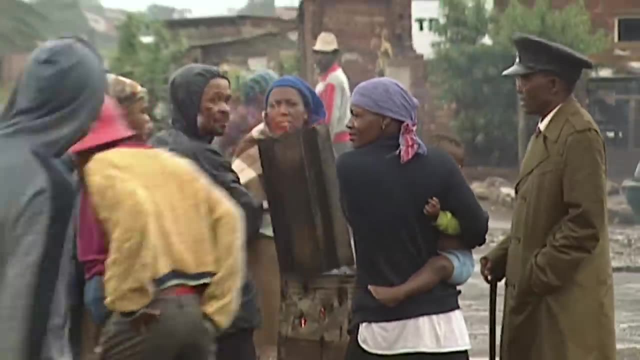 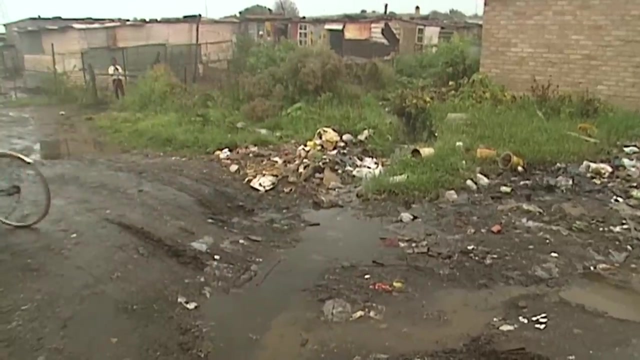 ESCOM officials who had, to this point, maintained an understanding that, as long as it provided cheap electricity- and lots of it… the state would keep its hands off. The paper, like the government that authored it, meant well—it properly identified the host of issues, but it pushed the longer-term problems to the back of the line and tried. 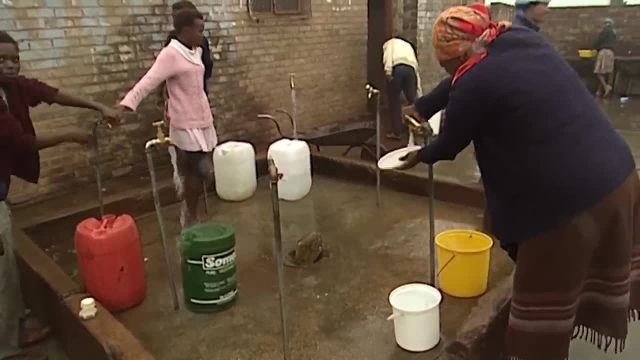 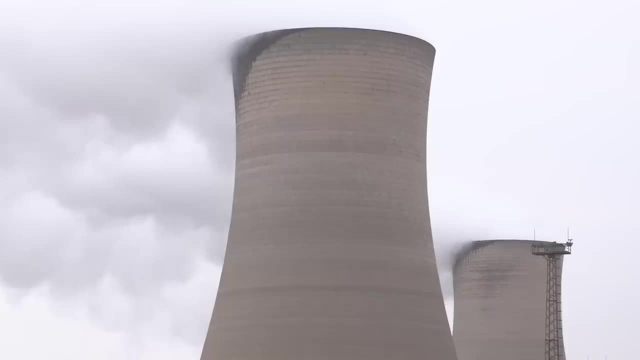 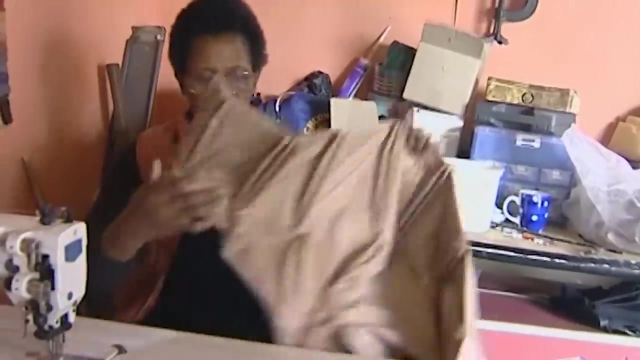 to radically reform through vague and confusing mandates With the grid and beyond it, there was just too much to get to. Some problems the white paper identified were addressed by the ANC as grid access expanded and pathways for black managers to work for the utility and black-owned businesses to contract with utilities were expanded. Some problems the white paper identified were addressed by the ANC, as grid access expanded and pathways for black managers to work for the utility and black-owned businesses to contract with utilities were expanded. Some problems the white paper identified were addressed by the ANC, as grid access expanded and pathways for black managers to contract with utilities were expanded. 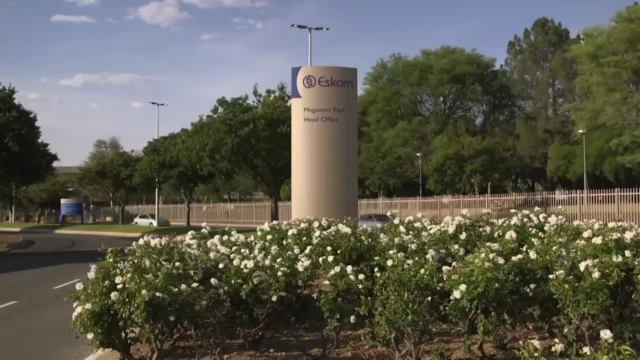 Some problems the white paper identified were addressed by the ANC as grid access expanded and pathways for black managers to contract with utilities were expanded. But other problems were only made worse as the ANC banned ESCOM from building new plants to stimulate competition. 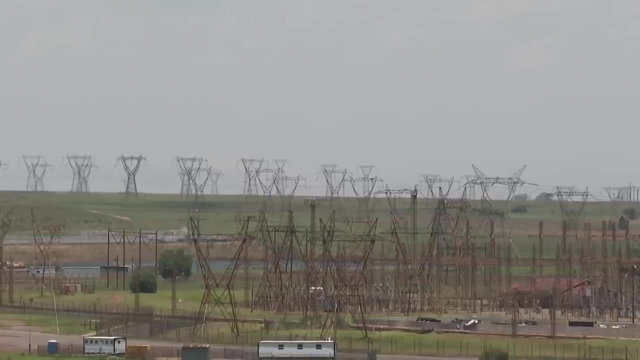 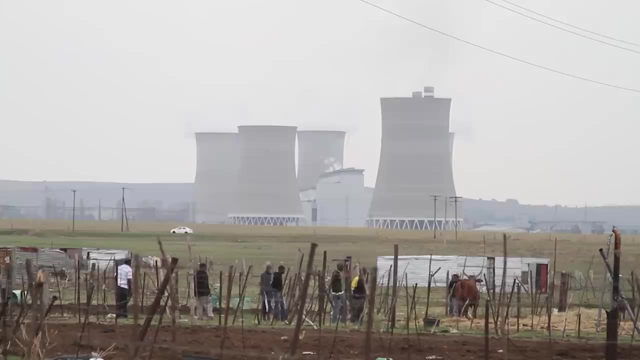 Ultimately, only when no competition appeared and the country began eating too far into its margin did the ANC reverse the ban. It was too little, too late by then, as the nation that had been known for its energy surplus, selling to nearby neighbors and producing megawatt-hour totals nearer to European. 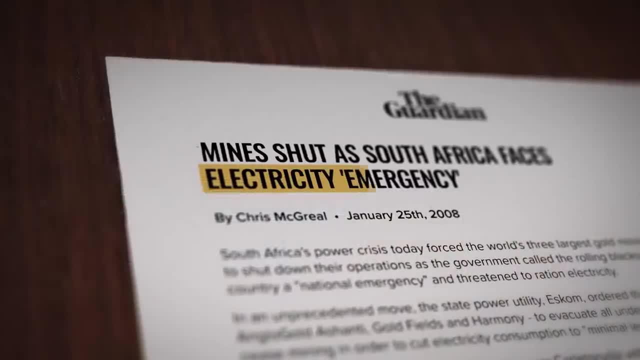 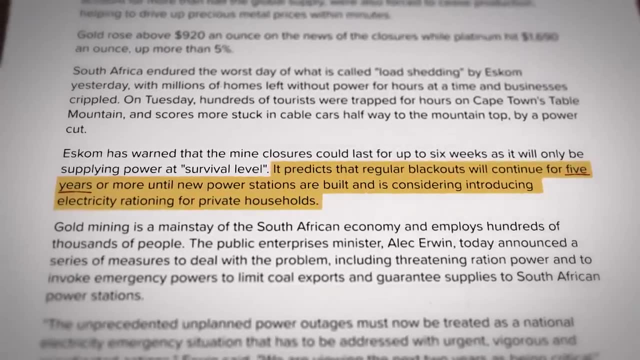 averages than those for its own continent, was now energy insecure by 2017., With experts saying that they wouldn't be able to dig themselves out of the hole for another five years. But more than 15 years on, as additional power plants have belatedly come online, the country's 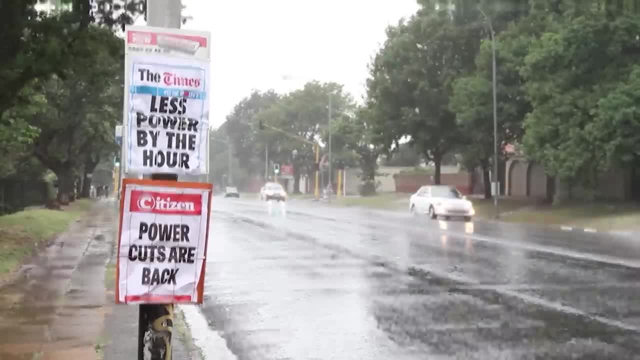 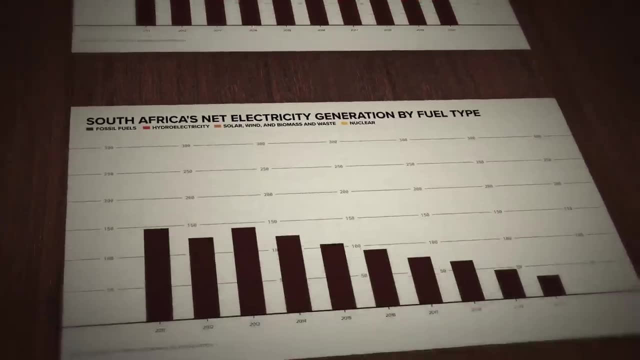 still in the grips of regular rolling blackouts. Across the 2010s, power capacity in South Africa steadily rose. The problem was actual production still stagnated. It's one thing to build the plants and another to keep them running. In late 2014 and early 2015,. the power plants were still in the market In late 2014 and early 2015,. the power plants were still in the market In late 2014 and early 2015,. the power plants were still in the market. 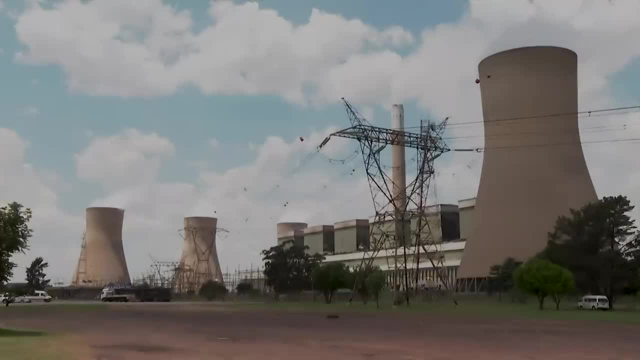 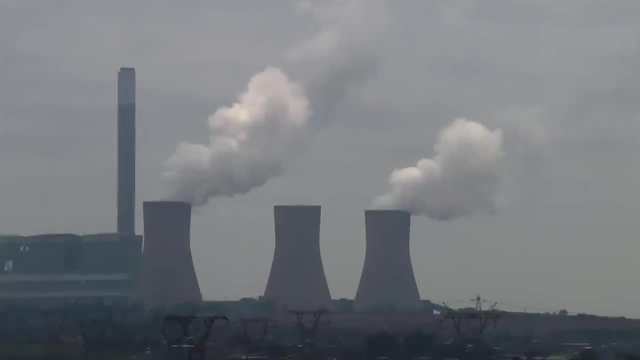 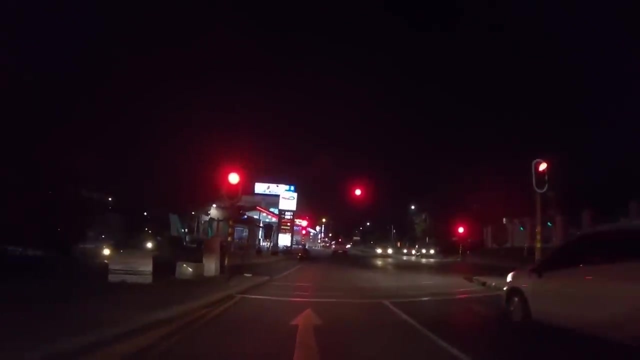 2015,. it was diesel shortages, drought and plant maintenance that cut national power production short of demand. In 2019, it was a coal shortage, flooding and alleged sabotage that led to worse blackouts. Finally, beginning with maintenance issues, in 2021, South Africa entered a spiral into 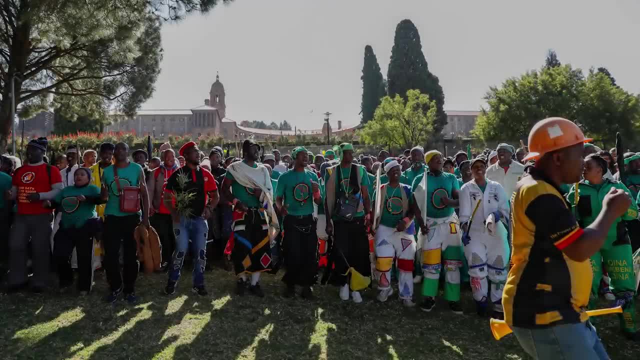 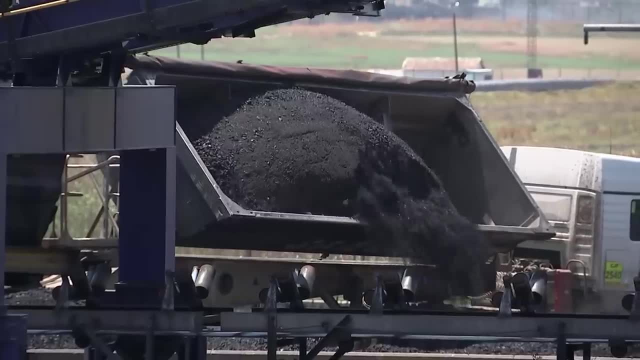 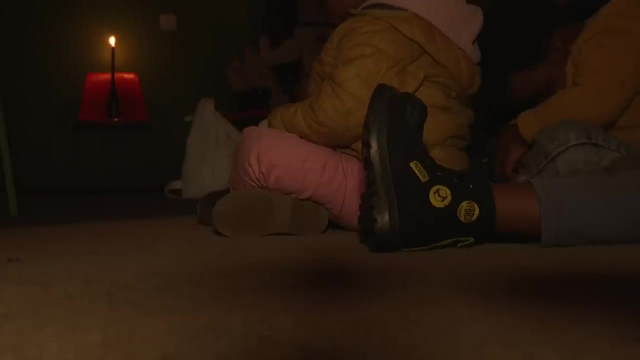 its worst outages ever: Employee strikes in June of 2022, fires and failures in September of 2022, then more plant failures in 2023 left some cities dark for entire days, while countrywide blackouts occurred at least once during 200 days of 2022—a new worst. Delayed maintenance, old coal plants and staff limitations were to blame, But so too was institutional rot. What was supposed to be fixed by ANC overhaul had fallen victim to the same ills, plaguing the ANC itself With cuts reaching 12 hours a day—. 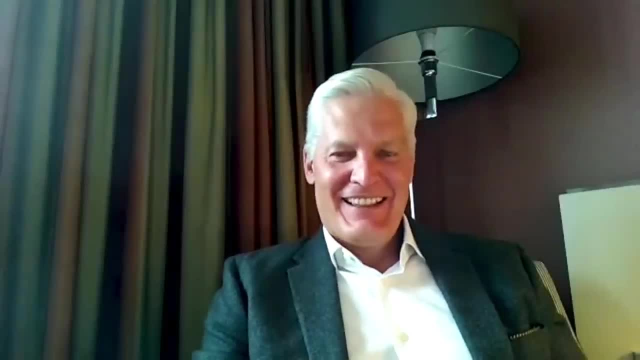 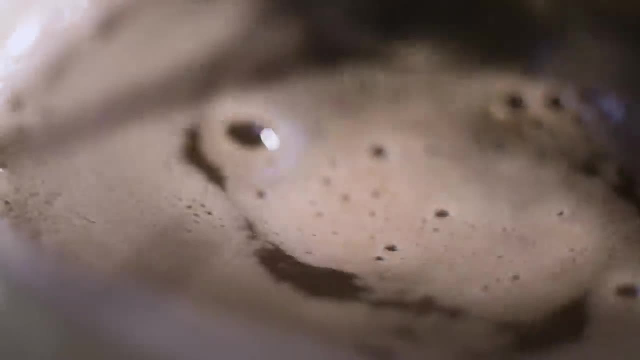 by the end of 2022—ESCOM CEO André de Reuter privately resigned- a move which nearly killed him- when, just hours after, someone slipped a potentially lethal doth of cyanide into his coffee. In a now-deleted interview revealing this close call, the former CEO went on to accuse: 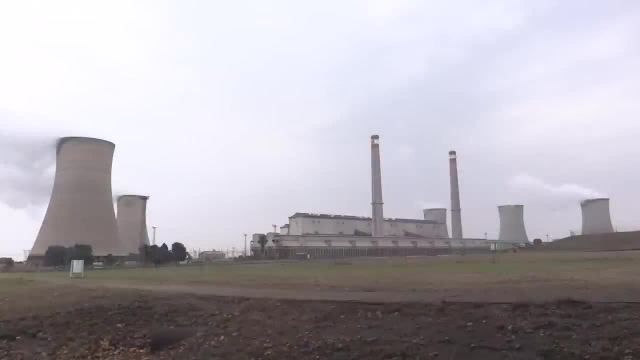 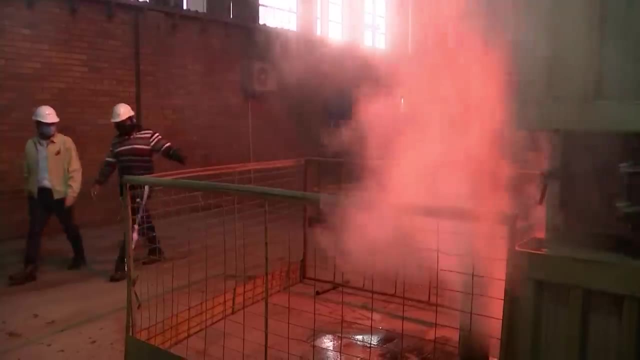 the ANC of institutional corruption, where ESCOM served as the feeding trough, with an estimated 1 billion rand, or $52 million, being stolen from the state utility every single month. While such a number is nearly impossible to find, the ANC is the only one in the United. 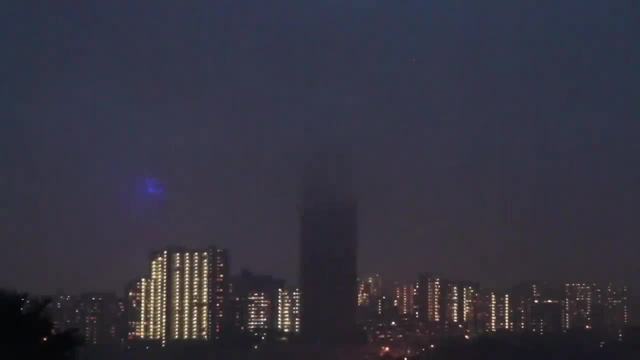 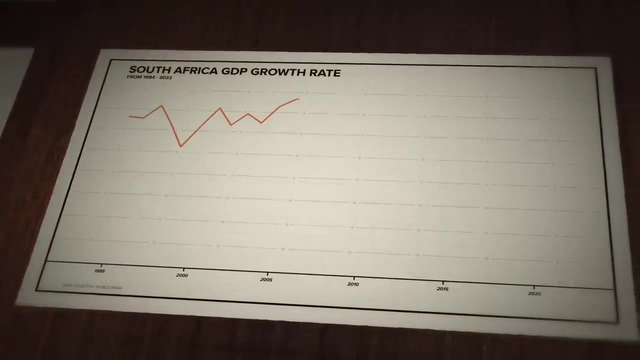 States that has the power to do so. While it is nearly impossible to verify, it would mark only the most direct loss that such widespread and long-lasting blackouts are creating. Post-apartheid GDP growth, which the ANC had once hoped to average 6% a year, has touched. 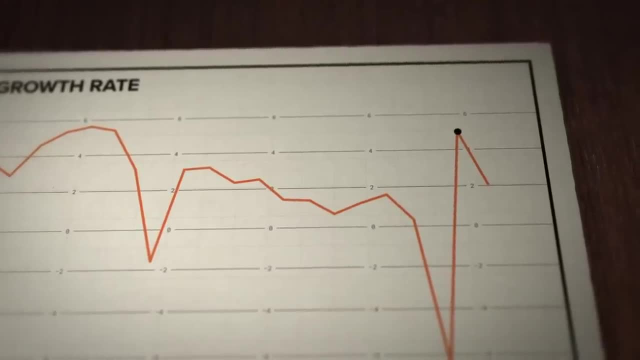 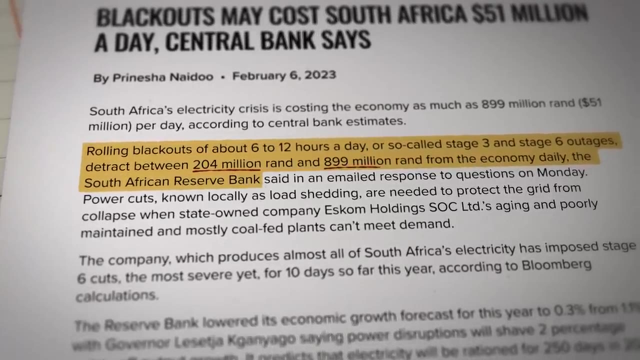 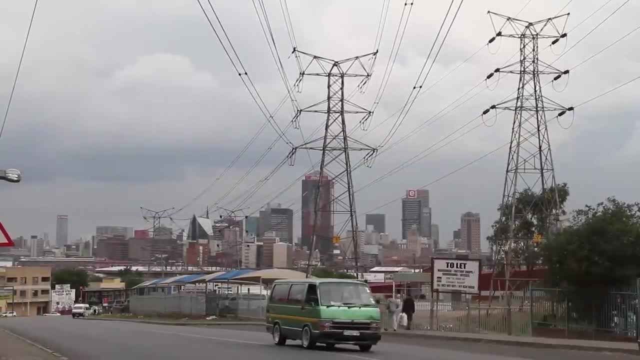 The ANC is the only one in the US that has the power to do so. The ANC is the only one in the US that has the power to do so. ESCOM, for its part, has raised electricity rates from the global basement, yet still. 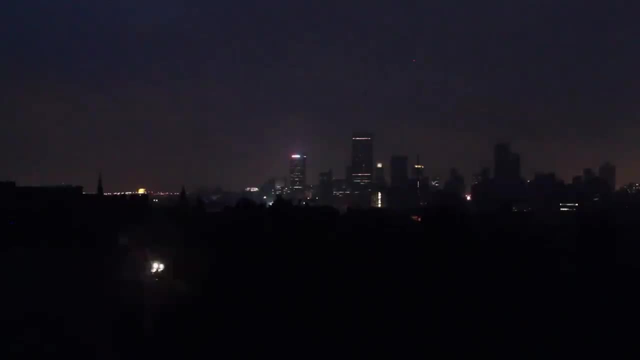 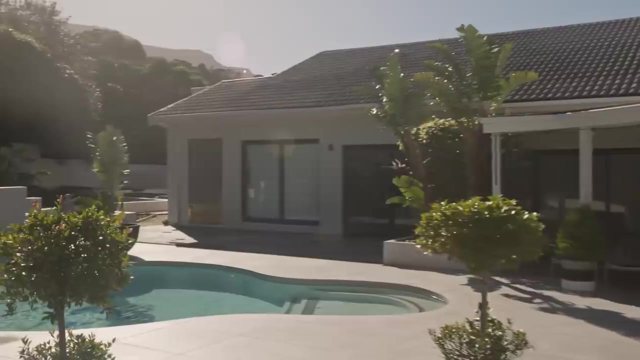 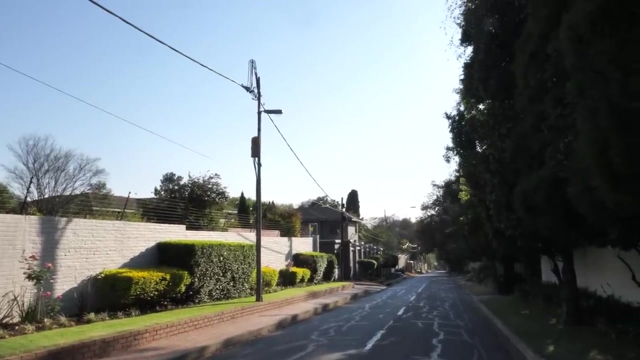 finds itself under a mountain of debt and unable to consistently keep the lights on. Confronting this darkness, nearly everyone, and everything that feasibly and financially can, are working to isolate themselves from the government, to build self-sufficiency from the public services that they can no longer rely on. 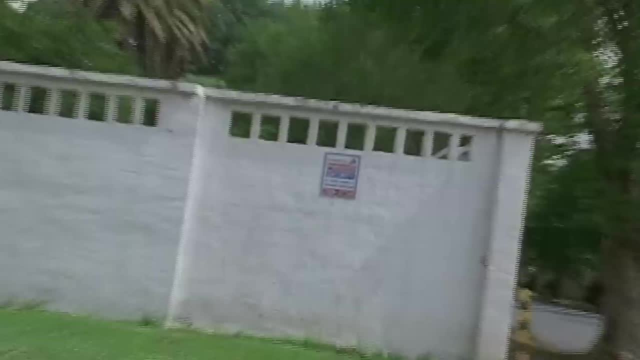 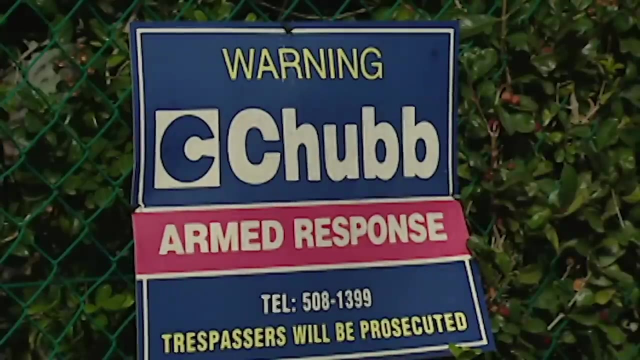 To start with police response times often stretching into hours. the wealthy rely on the world's most important resources- the most important resources—the public and largest private security industry- to keep them and their homes safe. More people are employed by this industry, in fact, than the police and military combined. 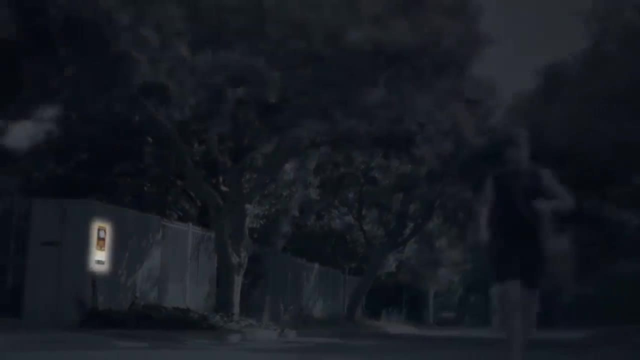 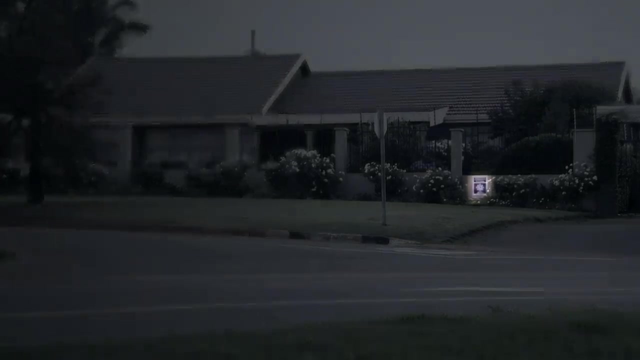 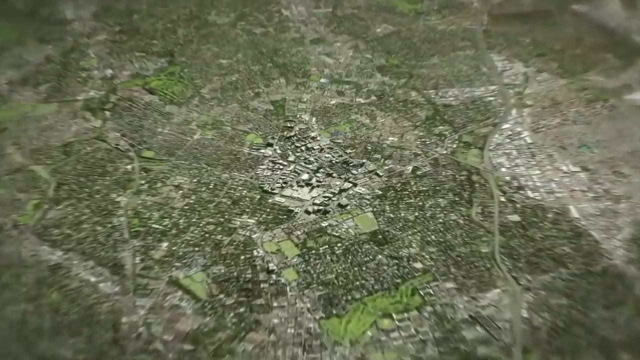 That's because nearly every expensive home is plastered with a plaque indicating which of the plethora of armed response security companies they're subscribed to, each of which patrols the nice neighborhoods and shows up far faster than the police Outside of their homes. the life of the wealthy has largely receded from urban downtowns into 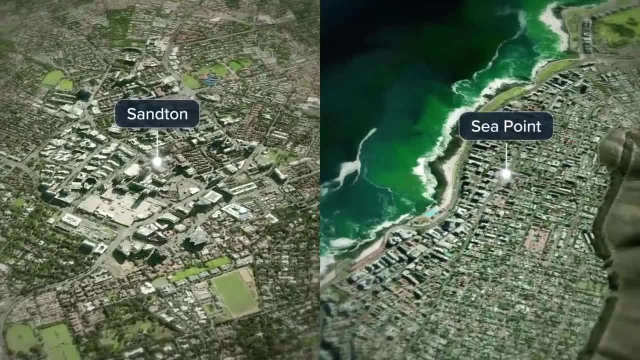 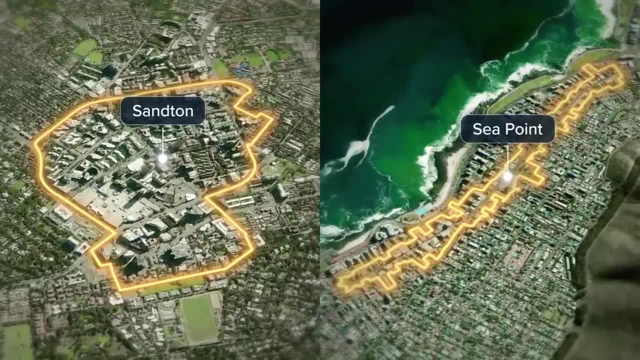 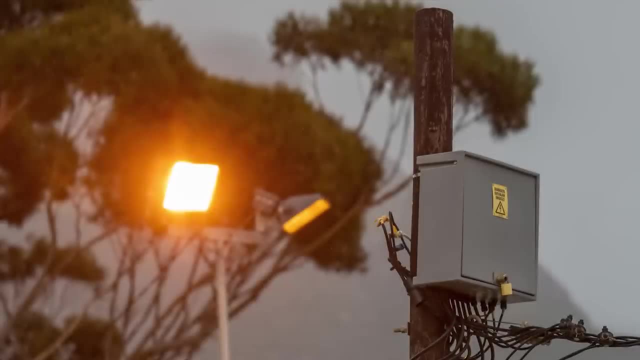 places like Sandton and Johannesburg, or Seapoint and Cape Town, both of which have organized into city improvement districts where the local private sector groups together and pays into an organization that ensures safety by hiring private security to patrol the streets. And some go further: filling potholes, fixing streetlights, cleaning litter, doing all the 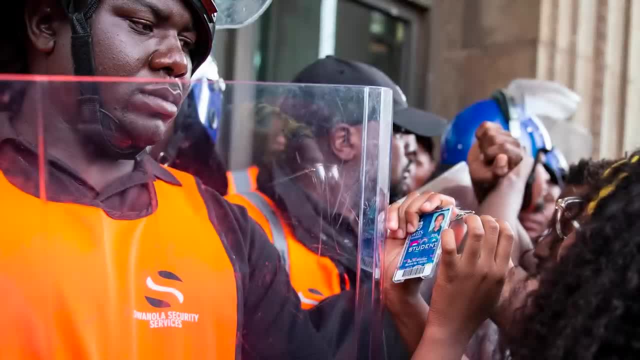 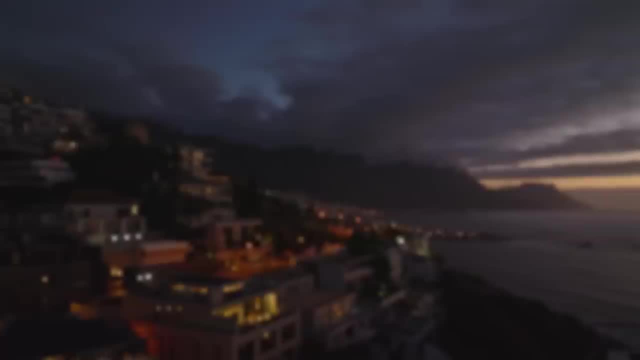 things that are the responsibility of the government on paper but that don't happen regularly or reliably in practice. In sum, the proliferation of private security and city improvement districts allows the wealthy areas of the country to maintain a semblance of stability, offering pockets. 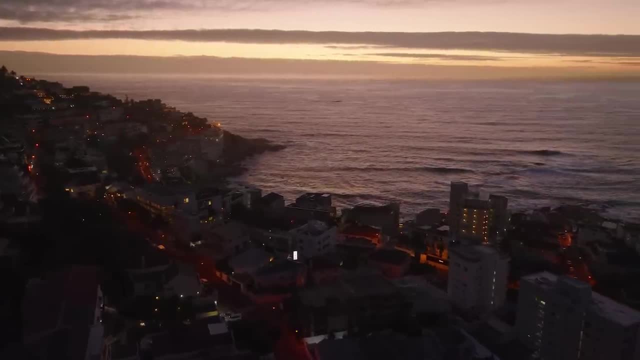 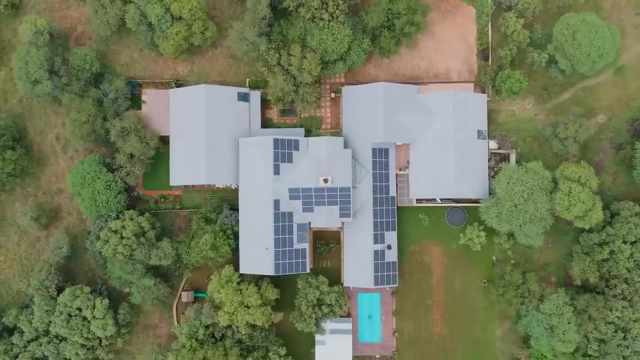 where the day-to-day experience is no different to that of Europe, for example. And this disconnect with their surroundings goes further for the wealthy few, as one of the nation's booming industries is now solar installation. South Africa's total solar capacity has more than doubled in just a year. as those 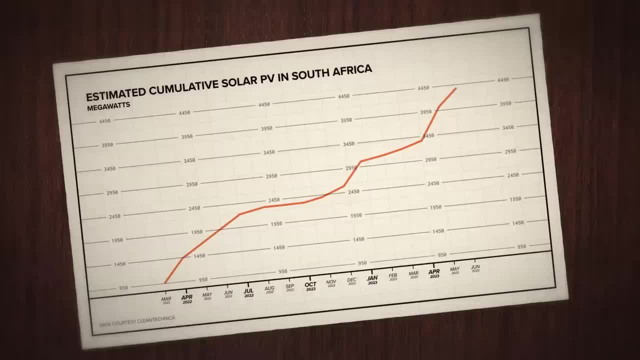 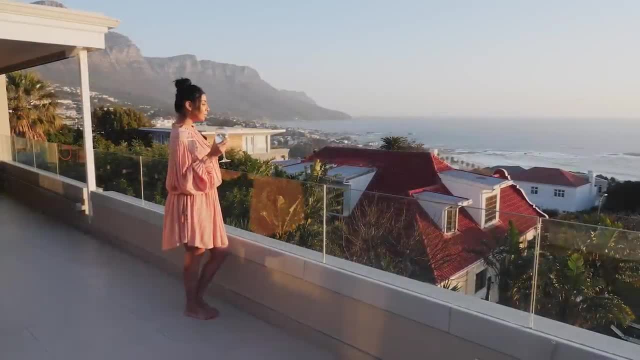 that can afford it are purchasing setups to allow for stable electricity regardless of grid conditions. And as perhaps the penultimate form before emigration, many wealthy people have been forced to leave the country and many wealthy residents are preparing to eliminate their reliance on the South African state entirely by gaining the right to live abroad. 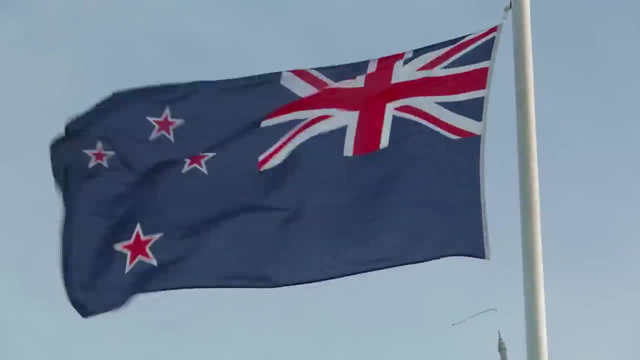 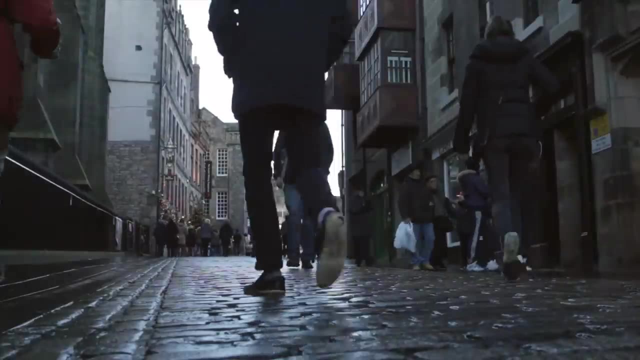 Those that can obtain Australian or UK citizenship based on ancestry are exercising those rights en masse, while immigration lawyers and nations are increasingly capitalizing on the fears of those that can't. Neighboring Namibia, for example, is developing a sprawling golf resort in Walvis Bay that 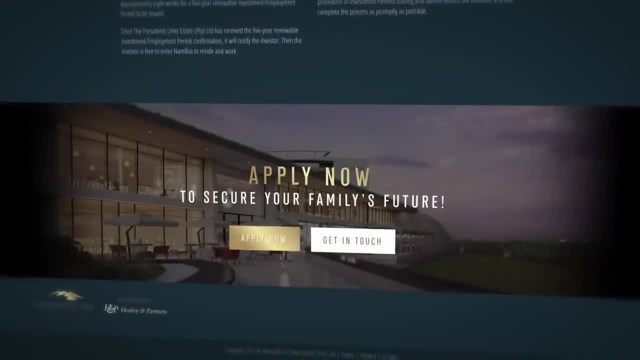 includes, with the purchase of a condo or home, a renewable work permit for the country. Malta, St Kitts and Mead are also developing a new type of work permit for the country as well. The United States and Nevis and others are straight-up selling citizenship in exchange. 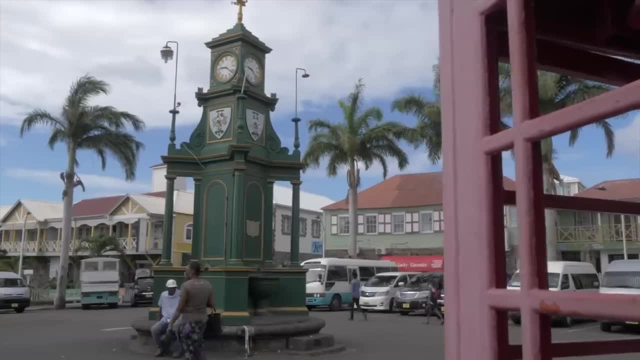 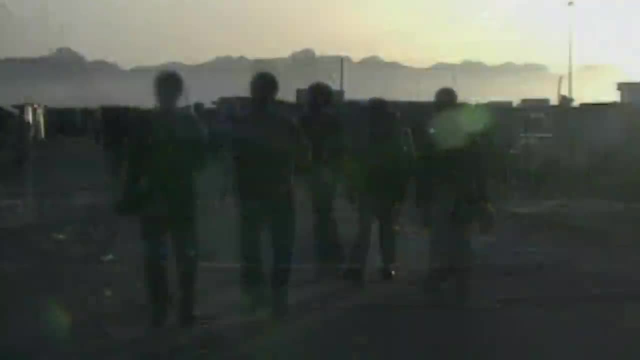 for six-figure so-called investments in the countries, and plenty of South Africans with the wealth to do so are taking them up on the offer in order to build out their Plan Bs Now. it's not like South Africa hasn't been in a similar state before. 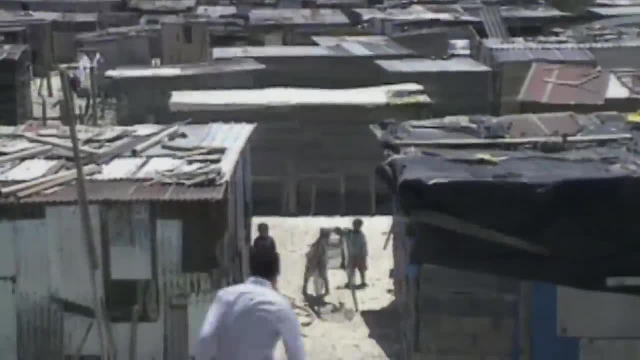 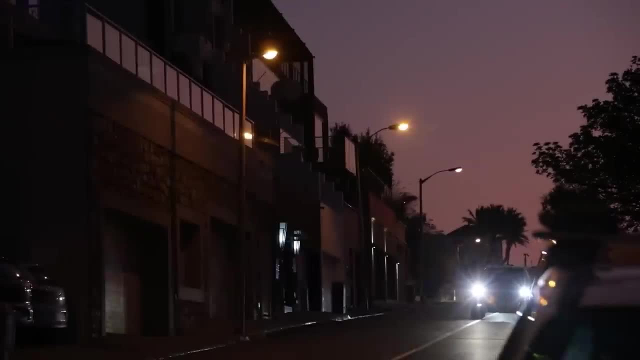 There was a time when crime was as high. there was a time when electricity access was worse. there was a time when, broadly, it was a less developed nation than it is today, but what makes its current reality so different is the fact that it's now a more developed. 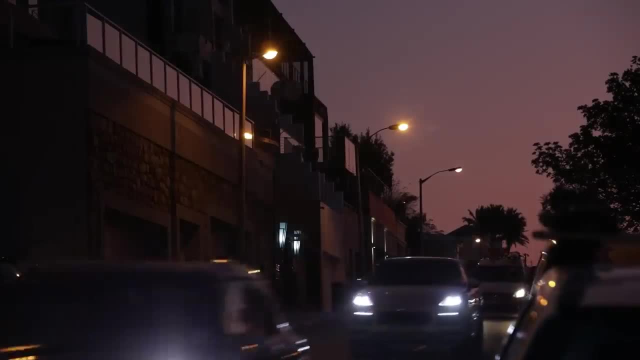 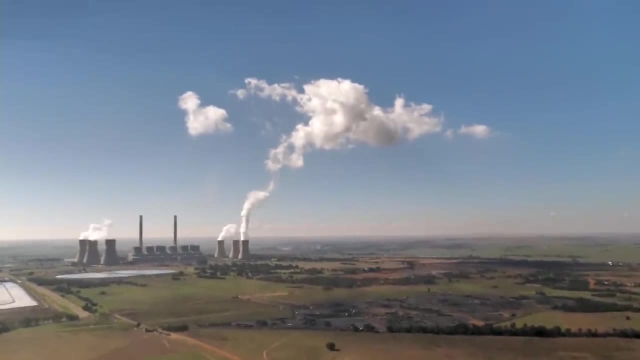 nation than it is today. What makes it so grim is that it's in a state of regression—it is devolving from its previous state as one of the continent's most developed economies, And this devolution is morphing into a death spiral. Look no further than the load-shedding 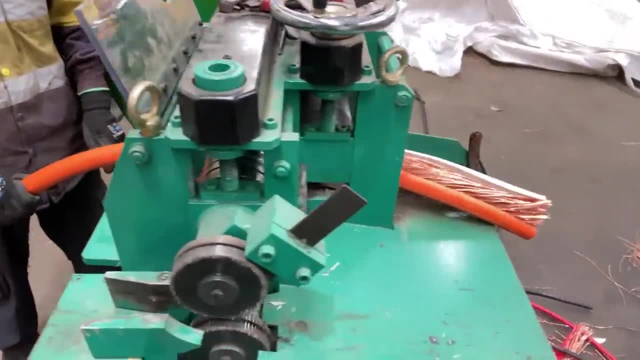 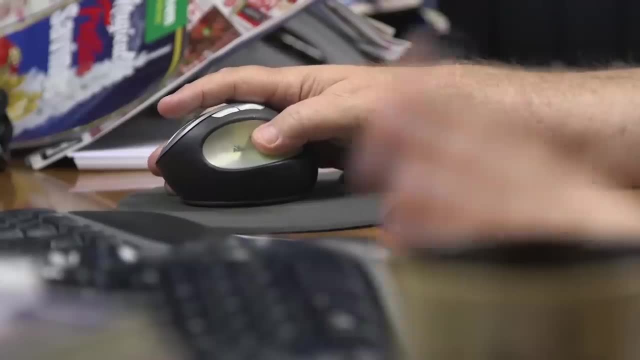 When the grid is turned off, the lack of dangerous electric currents makes it easy for thieves to remove copper cables and transformers. With each theft, the power utility has to divert resources towards fixing these new issues rather than the generating issues that are causing the blackouts in the first. 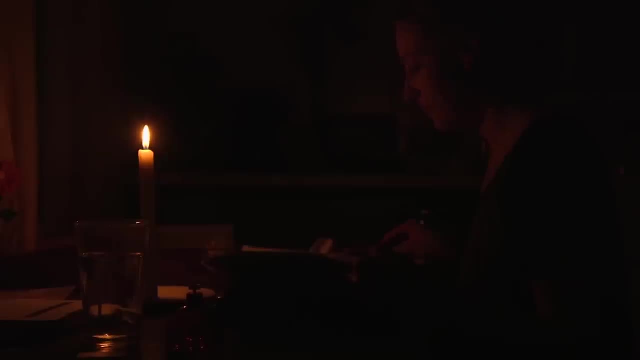 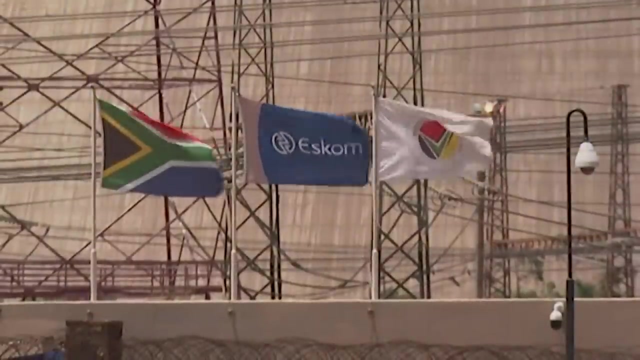 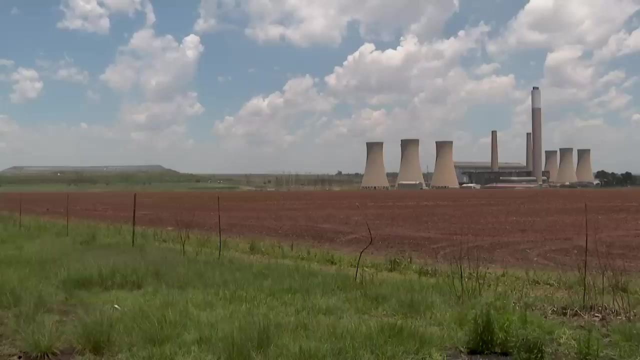 place. This makes the root cause worse, which makes blackouts more common, which makes theft more common, which makes the root cause worse, and so on. A certain degree of solution could come from the overarching government rather than simply within the power utility itself. but with each power cut, businesses lose money. 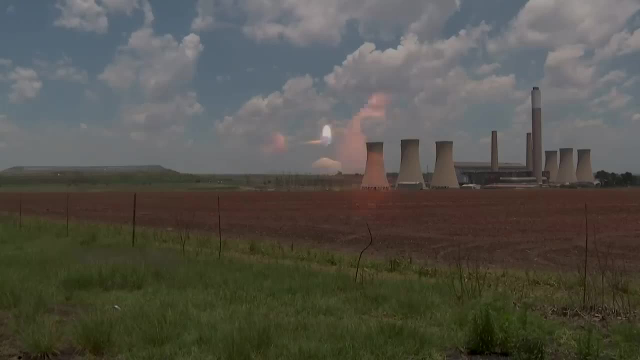 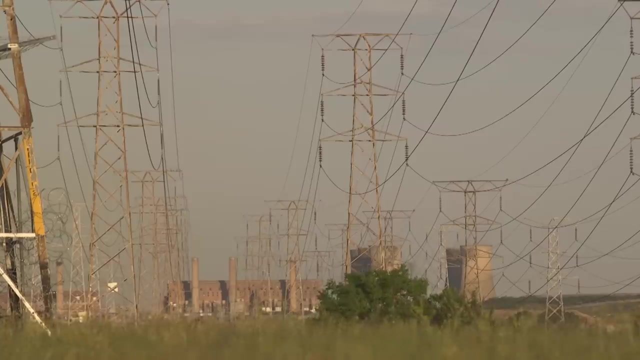 Production stops, food spoils, thieves, steal. The causes are myriad, but the effect is consistent—less income, which leads to a lower tax base for the government, which leaves it with less money to bring back around to solve the root cause, which makes blackouts more common, which makes the economic loss higher, which 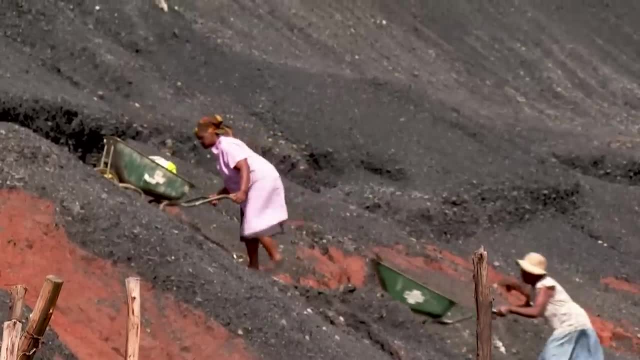 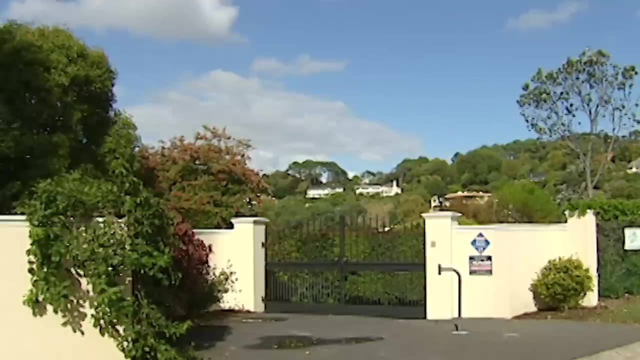 makes the root cause worse, and so on and so on. As all this occurs, quality of life declines for everyone in South Africa, even the wealthy few. They have to deal with higher crime, the inconvenience of load-shedding and a weakening economy. 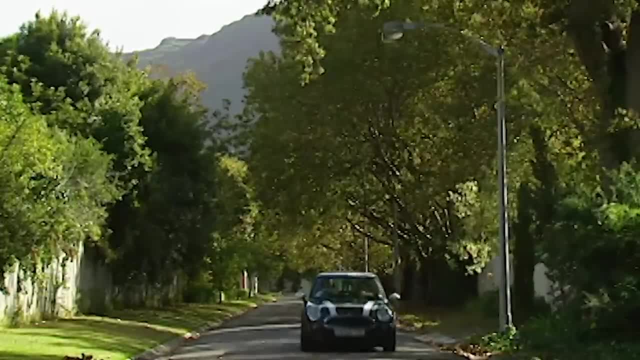 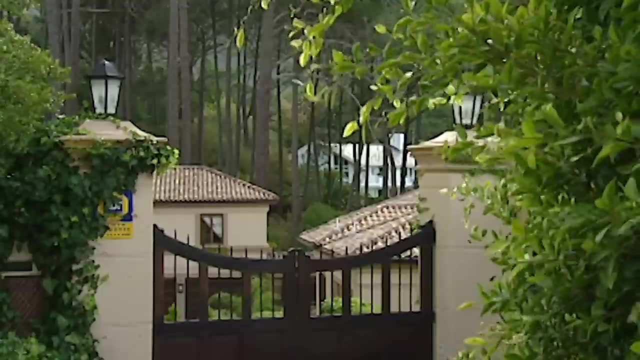 and rand exchange rate, which makes purchasing foreign-made goods and services increasingly out of reach. With the luxury of choice, the rich are emigrating, bringing with them their wealth, knowledge and business, which weakens the economy. The rich are emigrating. 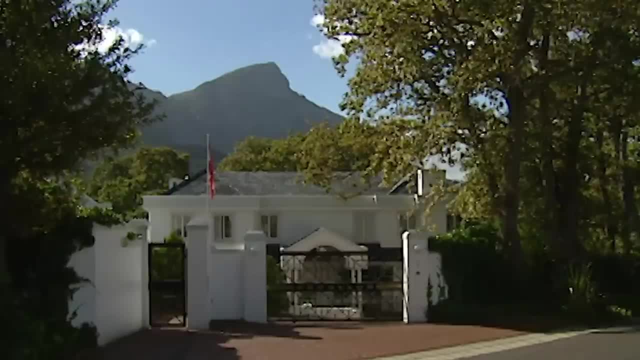 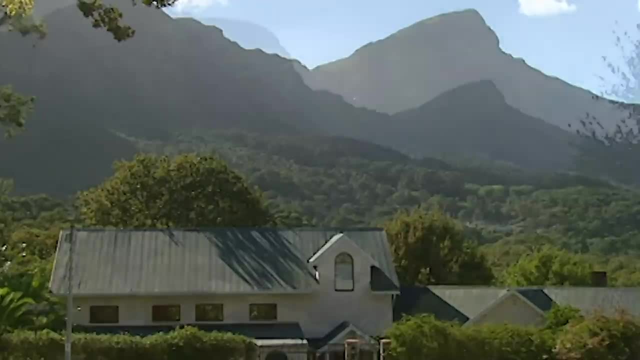 The economy, which makes the government less able to address the root cause, which makes blackouts more common, which makes more emigrate, which weakens the economy, which makes the government less able to address the root cause, which makes the root cause worse, and so on. 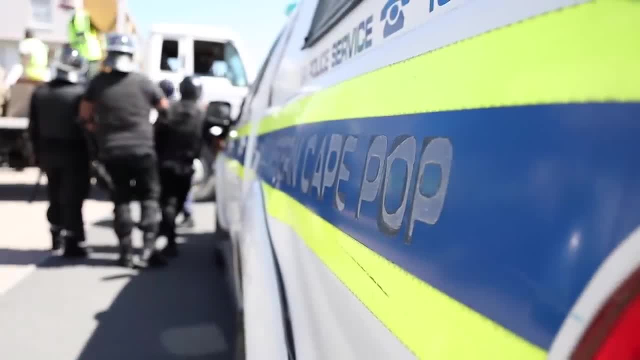 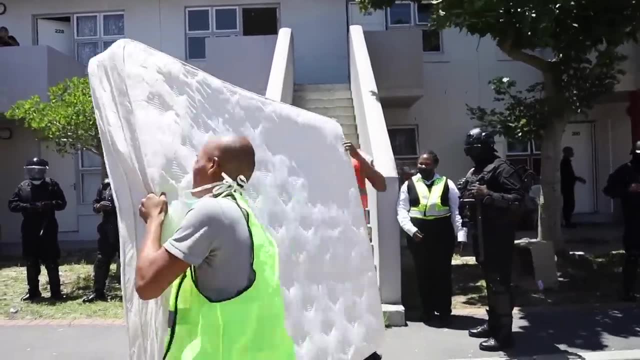 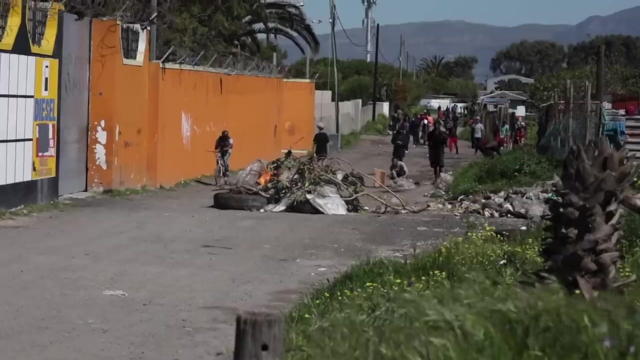 and so on and so on. This death spiral extends society-wide. It is now a central, unique, defining feature of the South African state. As the continent's poverty rate plummets, South Africa's is rising As the continent's human development rages. 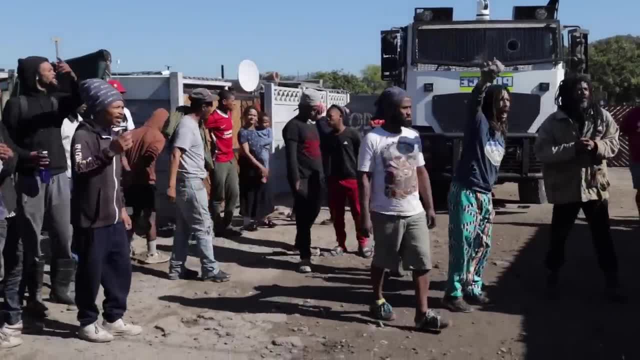 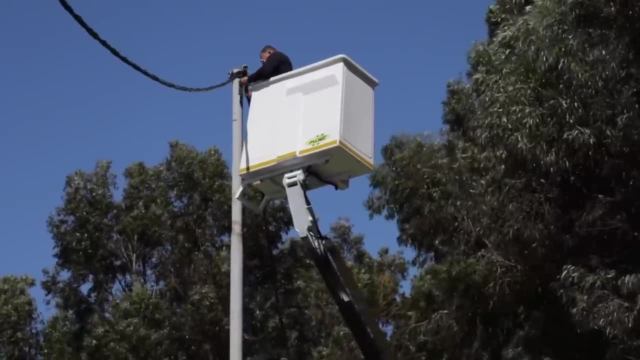 As the continent's human development rates go up. South Africa's declines. As almost every indicator of human and economic progress improves on the continent, South Africa's regresses. That's to say, this isn't some systematic issue, there isn't some force of nature. making the nation's decline inevitable, which leaves just one other possible culprit—the government. Support for the African National Congress, once synonymous with a support for the end of apartheid, has reached an all-time high. 2021 was the first municipal election that saw their share of the national vote drop. 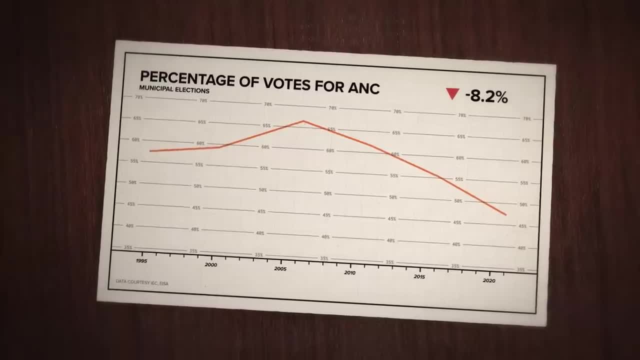 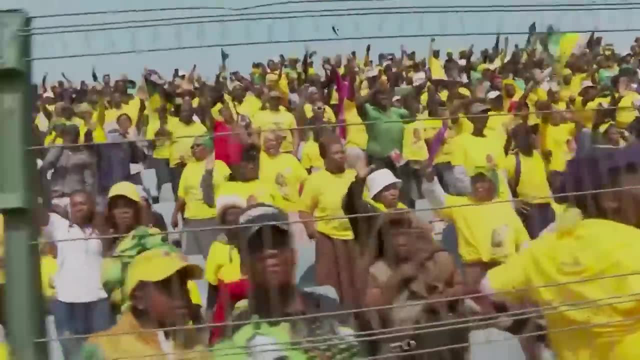 below 50%—essentially, every issue has only escalated since then, and new stories of corruption and cronyism within the party emerge every day. In 2024, the nation will elect a new National Assembly and, with declining support and 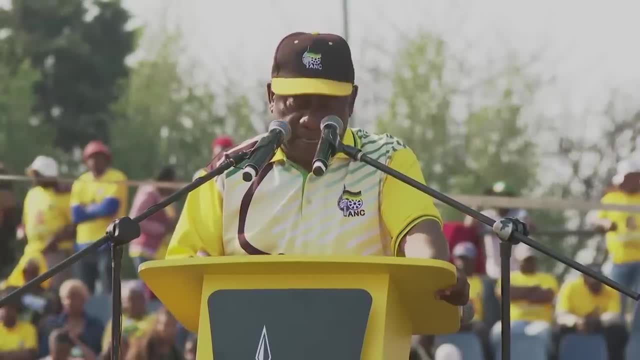 a growing coalition in opposition. the ANC is on its most tenuous footing ever and the country could see functional political plurality for the first time in a decade. The ANC is on its most tenuous footing ever and the country could see functional political 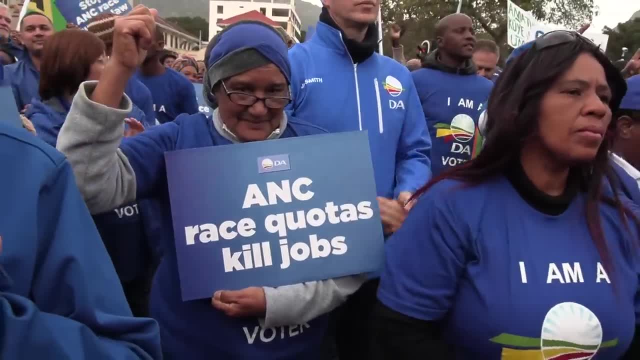 plurality for the first time in a decade. The ANC is on its most tenuous footing ever and the country could see functional political plurality for the first time in a decade. The ANC is on its most tenuous footing ever and the country could see functional political. 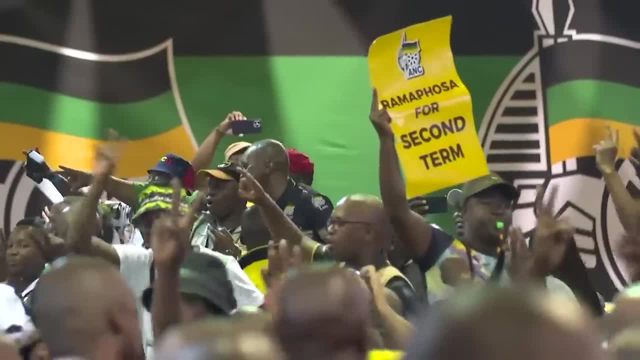 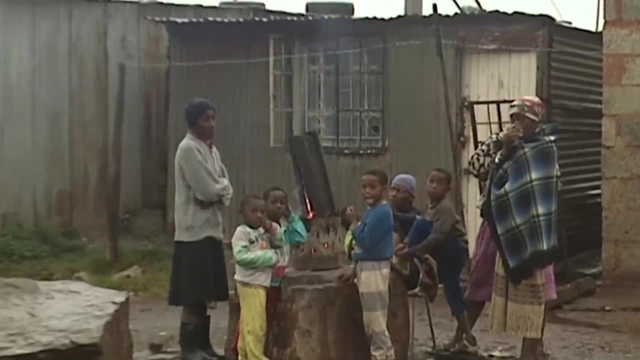 plurality for the first time in a decade. Now, as rhetoric focuses on whether South Africa will slide into failed state status, there is a question worth asking on whether the nation has ever actually been a functional state. There was a time when it seemed more stable and prosperous than today, but that was only. 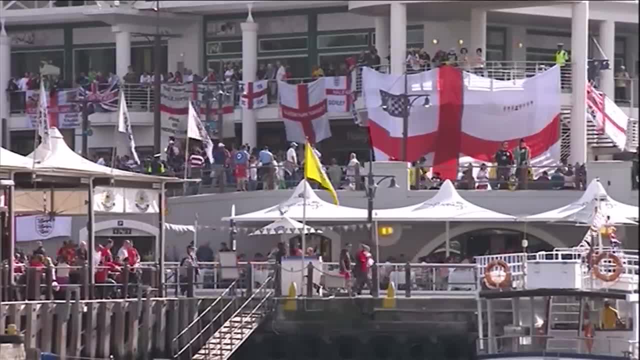 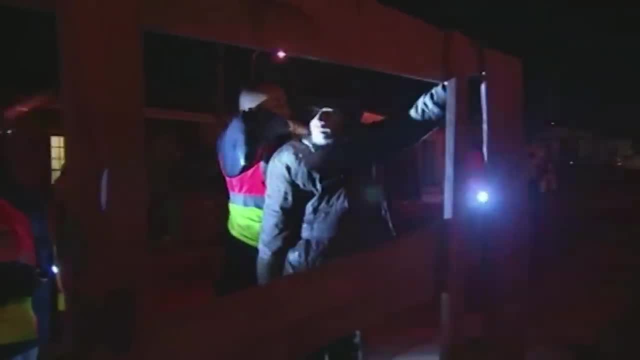 the part of the nation that one saw on World Cup broadcasts, the part lived in by South Africans one would meet abroad—more specifically, it was the white nation. while the black nation's voices were stifling Through the Apartheid era, South Africa failed to provide basic services of an acceptable 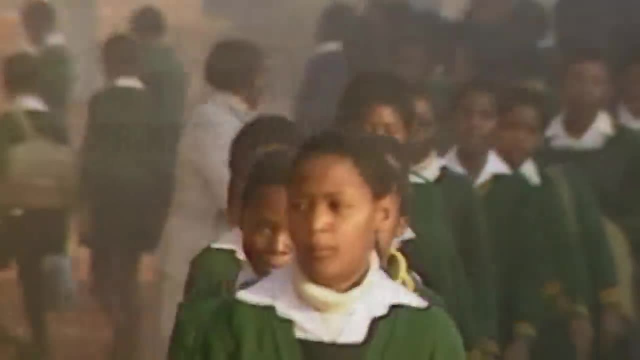 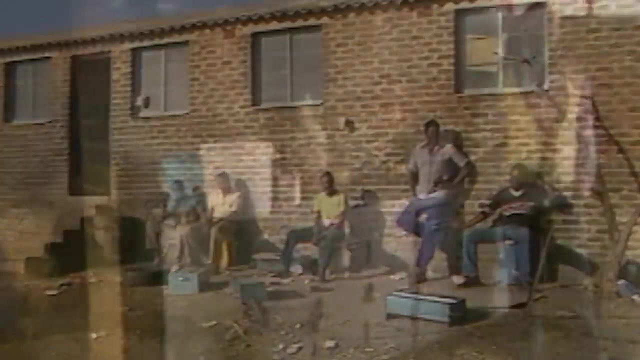 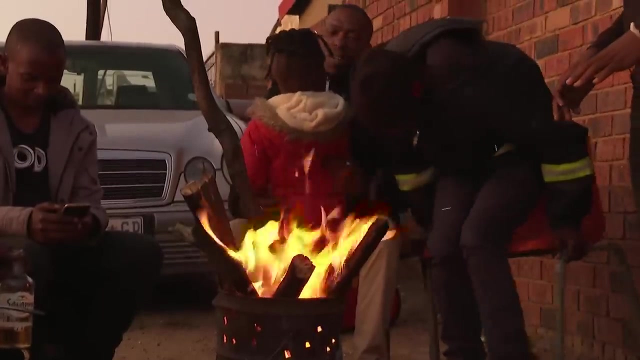 standard—sanitation, education, police—to the majority of its population—the black population. By many definitions, that is a failed state. So that's to say, basic services have never been at an acceptable level. The difference is that today the deficiency is being shared more equally. 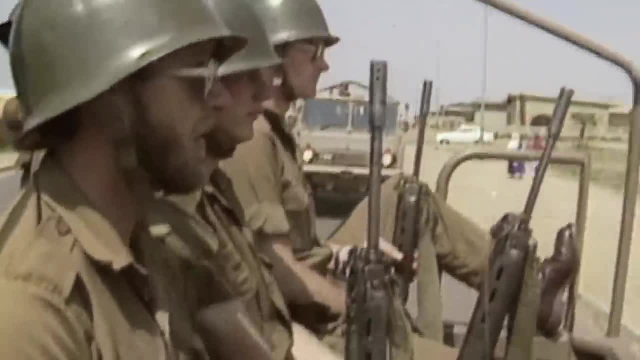 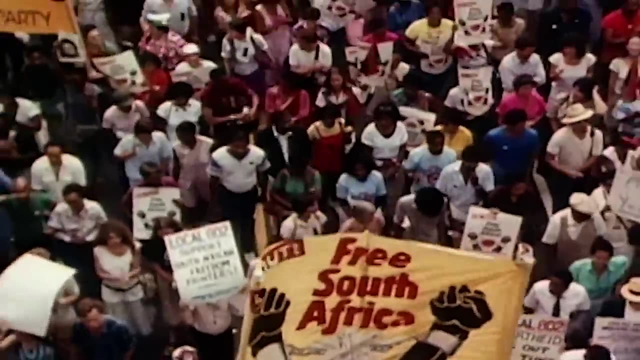 It would have been unrealistic to expect that a standard of living experienced by a privileged minority, propped up by oppression itself, could immediately extend to all—it was always going to be a tricky transition, But tragically, the ANC- the institution most responsible for inciting this transition- 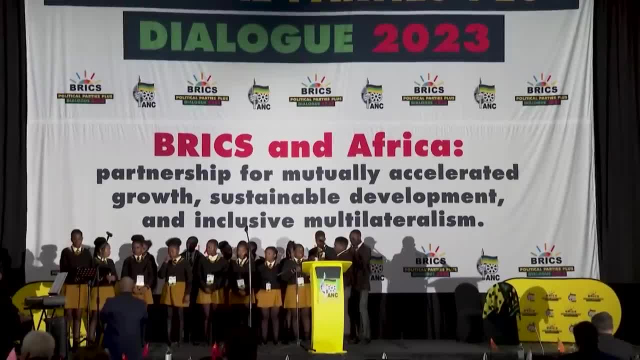 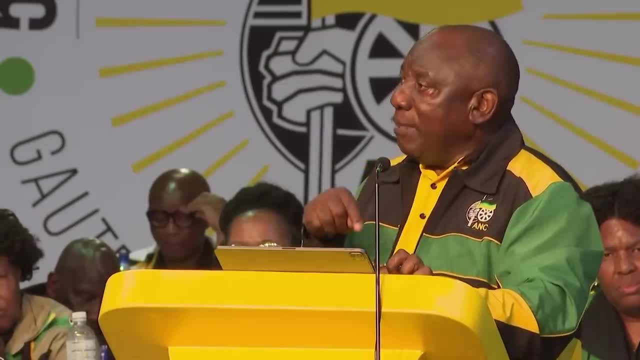 is now slowing it down. Party members are using their positions to steal from the state, to use oppression to prop up the privileged—the very dynamic they fought to end. Perhaps the sole light in the situation is the fact that it has worsened enough that. 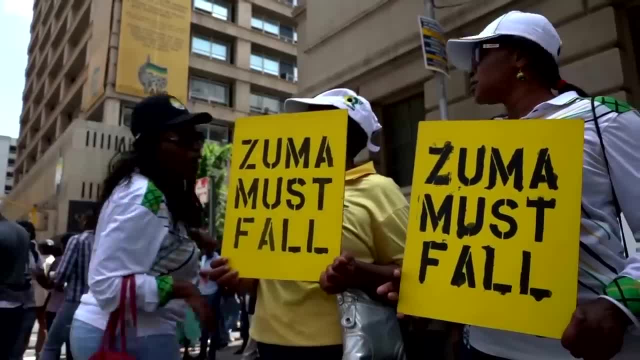 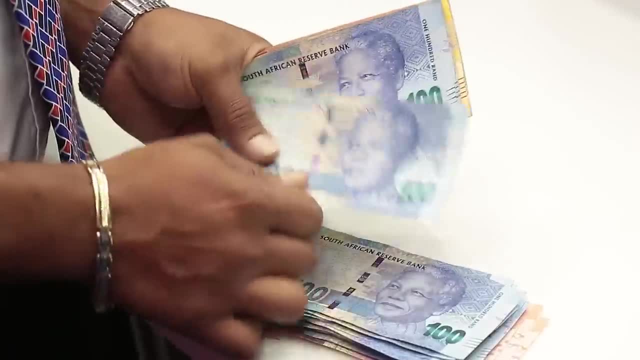 one can identify that the transition is failing—that a new approach is needed. South Africa still has a starting point that would be the envy of most of its continental neighbors. It still has a robust economy, a relatively high standard of living and is naturally 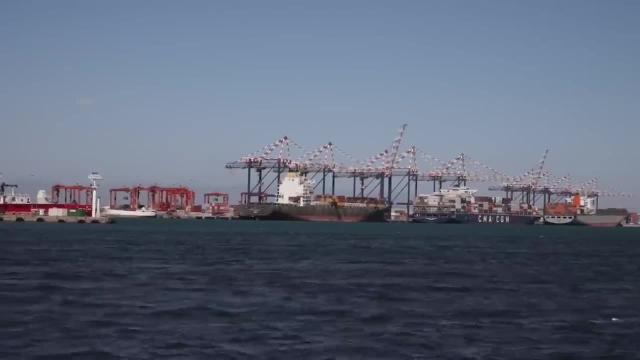 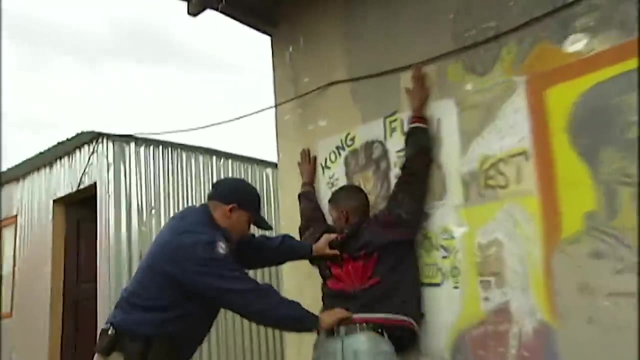 indebted with valuable resources, so it's not too late to capitalize on its situation and create a thriving state that truly works for all. but the window of opportunity is slowly starting to close With each passing day. those with the luxury of choice are…. 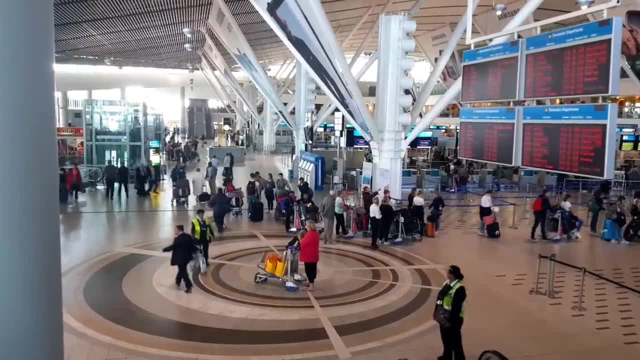 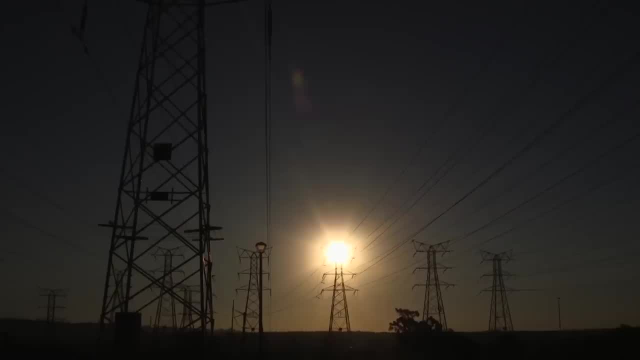 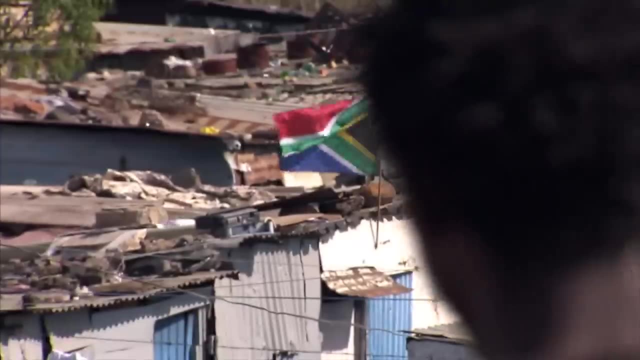 giving up. They're packing their bags and driving to the airport one last time. With each hour of load-shedding, the economy shrinks further and the death spiral accelerates. Hope is not lost in South Africa, but with each day that passes the path towards prosperity. 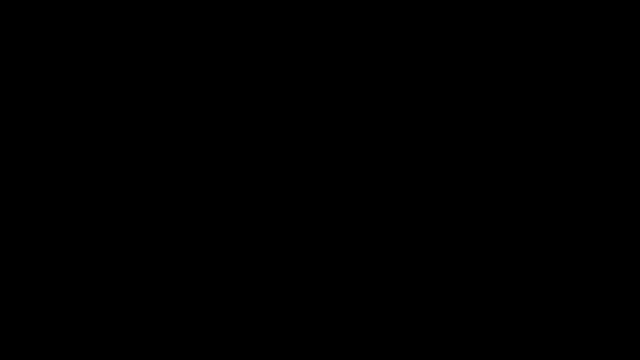 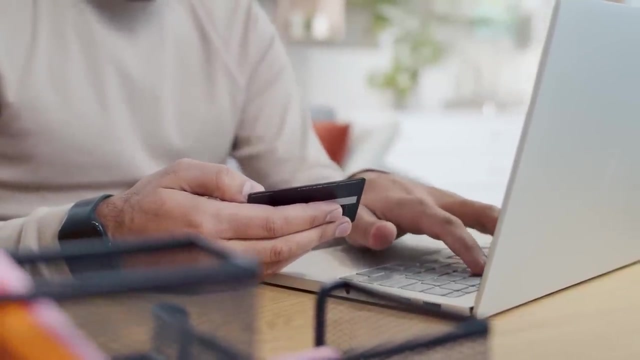 grows ever harder to find. Finance is tricky—it's a very easy thing to lose track of, especially as companies increasingly design their services around you for getting your spending. It's a very difficult thing to lose track of, especially as companies increasingly design their services around you for getting your spending. 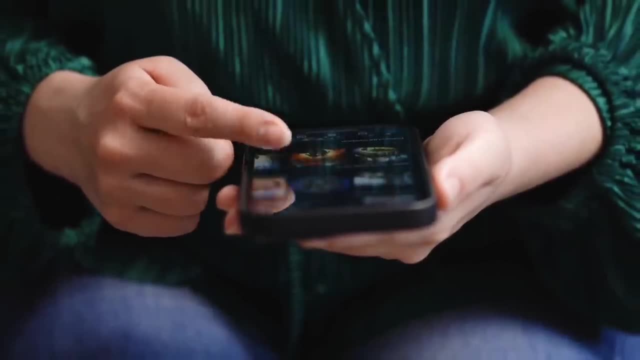 It's a very difficult thing to lose track of, especially as companies increasingly design their services around you for getting your spending. Subscriptions, especially, can really add up. but to help me manage my monthly spending, I recently started using our sponsor, Rocket Money. They're an all-in-one finance platform that helps you save more and spend less. Personally, I find it super useful, as they save for a down payment on a house, as I can build my custom budget that automatically monitors my spending by category plus monitor. 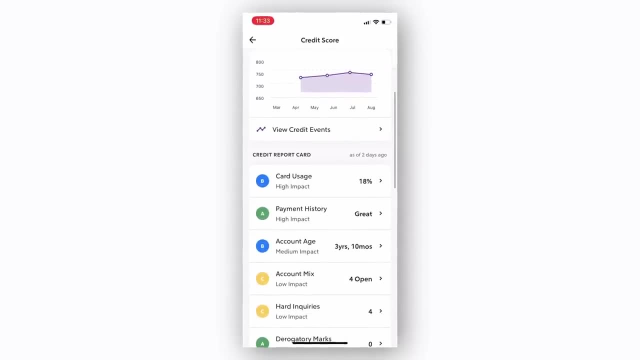 my credit score to make sure I raise it as much as possible to get a good interest rate, and it even allows me to automatically deposit a certain amount of money into a smart savings account to grow my business. Personally, I really like having Rocket Money as my all-in-one solution to money management. 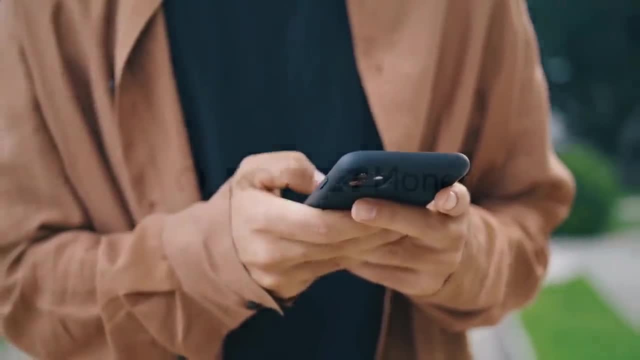 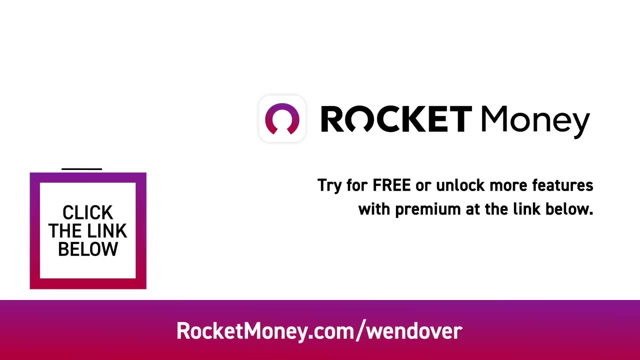 rather than having to use a bunch of different apps that don't really work together. and if you happen to be one of those very common people who want to save more and spend less, you can go to rocketmoneycom, slash Wendover or click the link in the description to get. 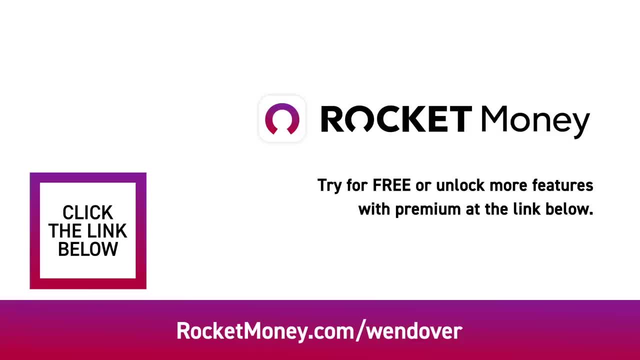 started for free, and then you can unlock even more features with Premium.